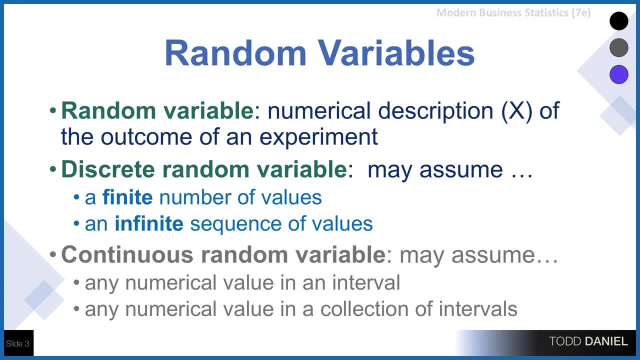 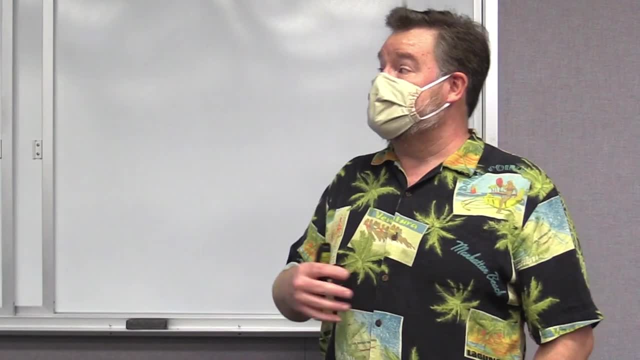 two kinds of random variables that we're interested in: The discrete random variable, which may assume either a finite number of values or an infinite sequence of values. And before I unpack that, I'll also mention the continuous random variable, which may assume any numerical value in an interval. 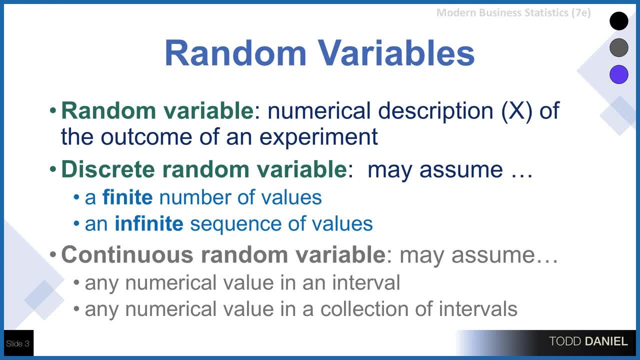 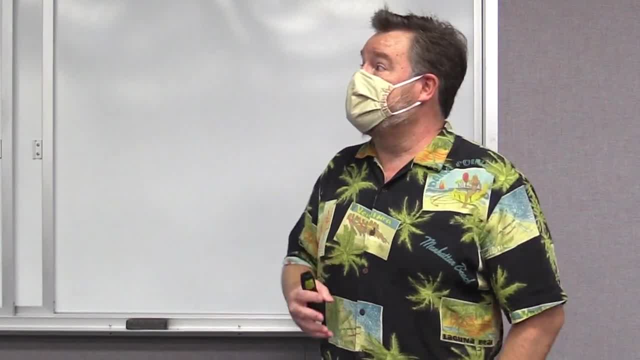 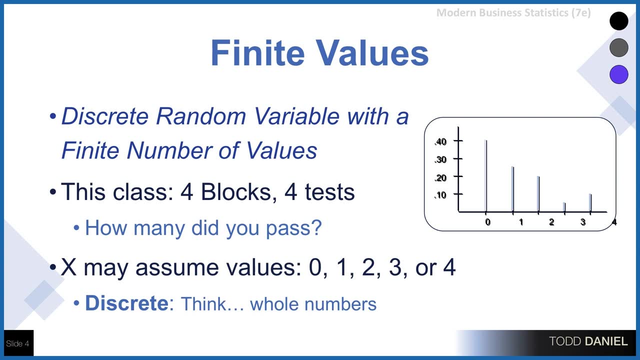 or any numerical value in a collection of intervals. That will be our topic for next week. So this week we're only going to focus on those discrete variables. And let's start with a discrete random variable with a finite number of values. Perfect example: this class. So you know we have. 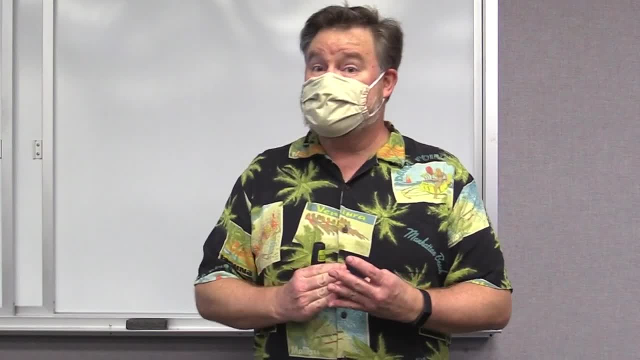 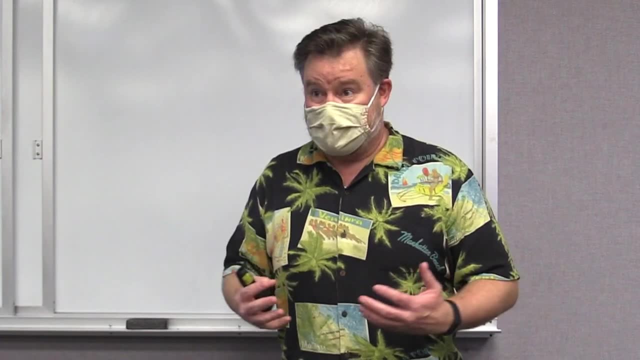 four blocks in this class and each block ends with a number. So we're going to start with a test. So if I ask, how many did you pass? The options are 0,, 1,, 2,, 3, and 4.. I could also ask. 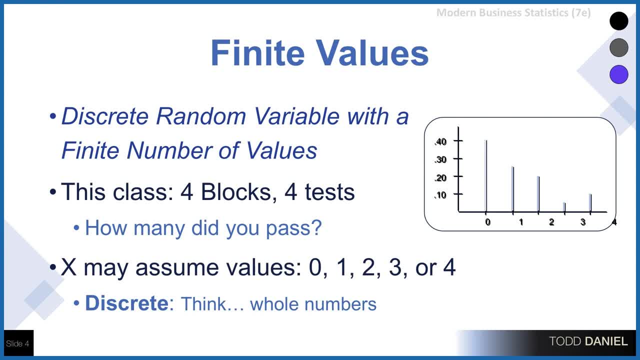 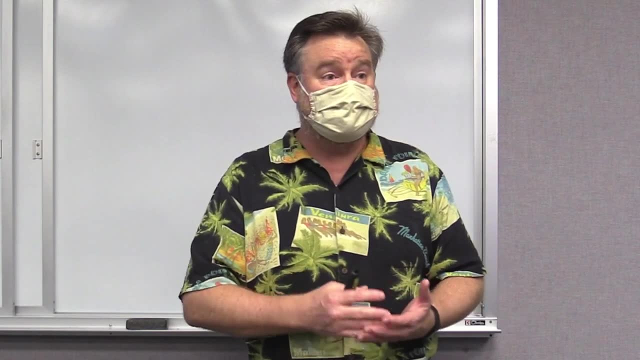 how many did you get an A on? Or how many did you get the grade that you were hoping to get? Or how many did you get at least a C? I could structure the question in multiple ways, but no matter how I structure that question, the answer- options are always. 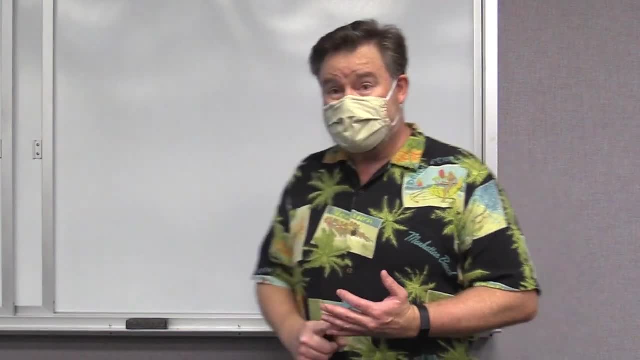 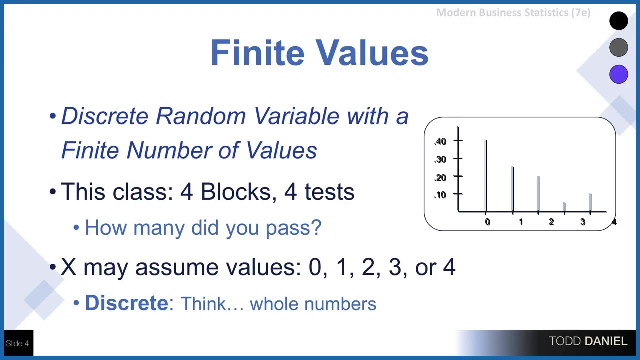 going to be the same: 0,, 1,, 2,, 3, and 4.. So when you think about a discrete variable, think of whole numbers. The numbers can only be whole numbers. You can't have passed 1.3 of the. 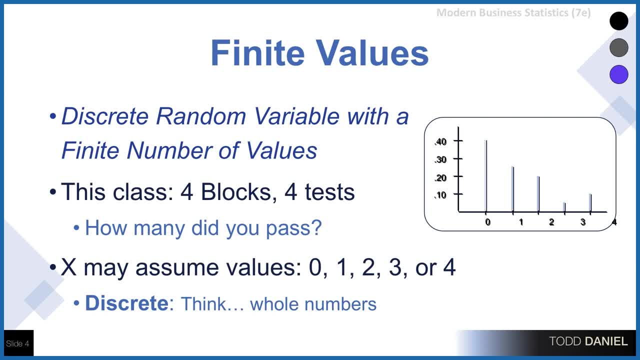 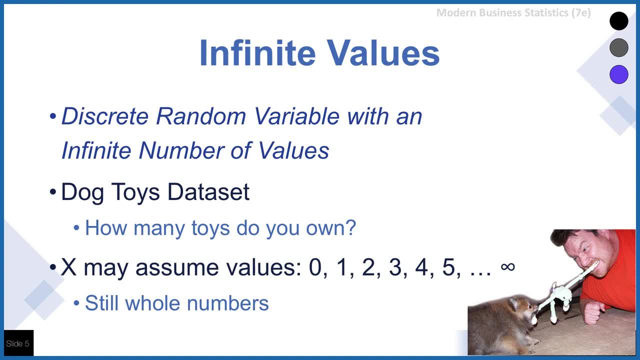 tests, You have to pass a value that is represented by whole numbers. A discrete random variable with an infinite number of values could be something like our dog toys data set. So remember, one of the questions that was asked was how many toys did you get? And the answer was how many toys did. 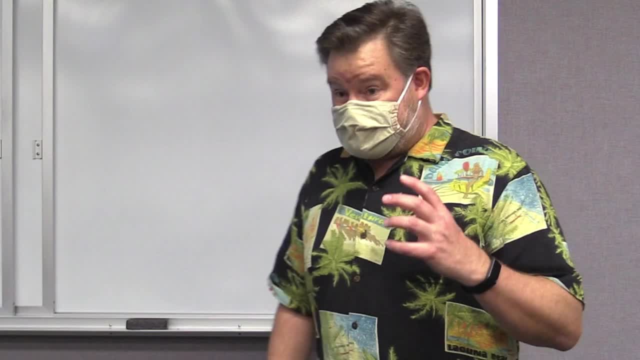 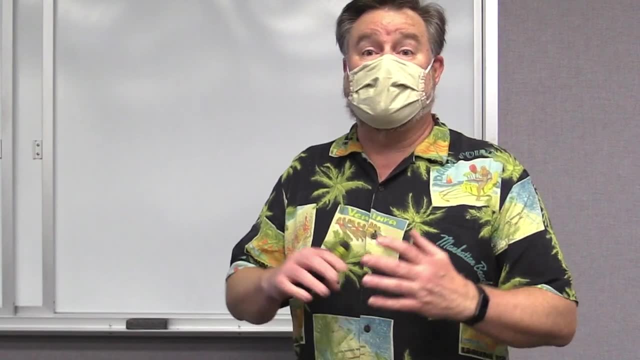 you own. It's still going to be whole numbers. However, the values could be 0,, 1,, 2,, 3,, 4, 5, but there's no upper bound. Certainly, that is defined by the question. It could, theoretically. 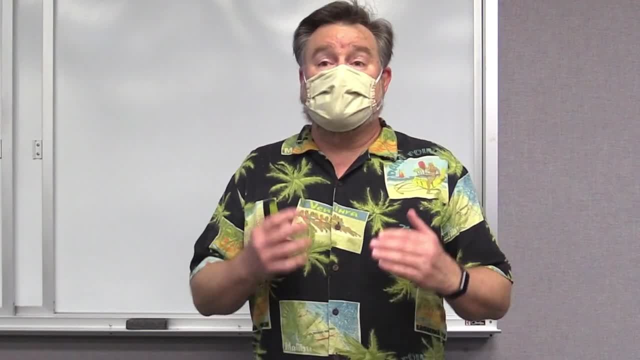 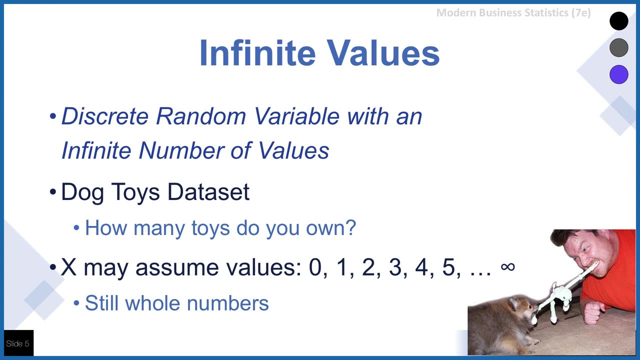 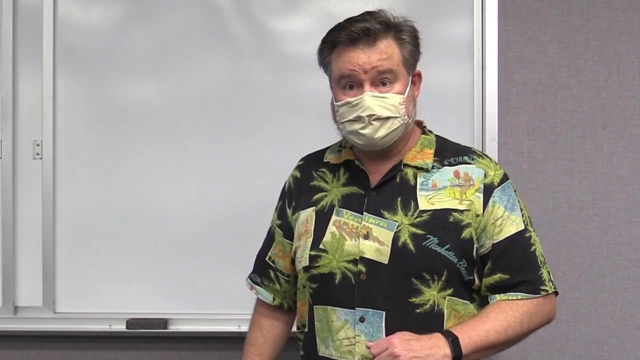 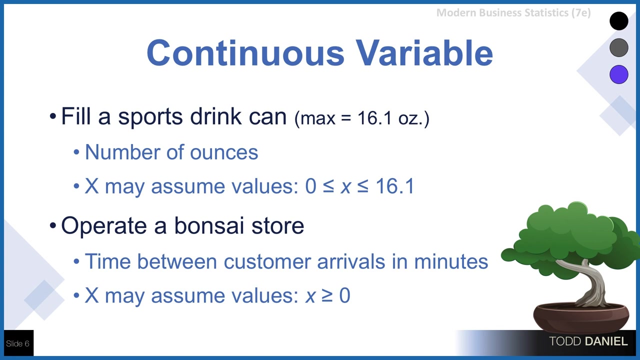 go to infinity. So we're going to be using whole numbers in any type of discrete probability distribution, And those values may or may not have an upper boundary, Which is what qualifies them as either being finite or being infinite. A continuous variable- and again this is our topic for next week- could be something like filling up a sports drink can. 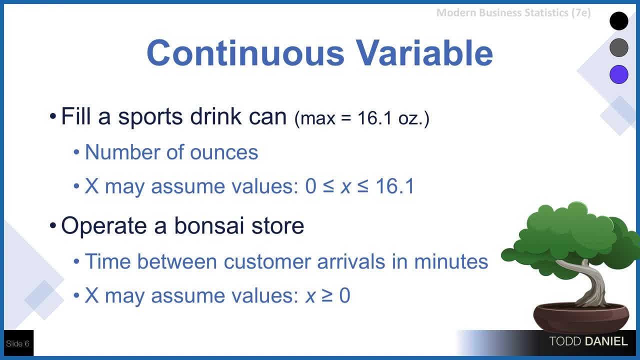 How many ounces of fluid are in the can? The maximum, according to the machinery, is 16.1 ounces. So how many ounces are in the can? Theoretically could range from 0 all the way to 16.1.. 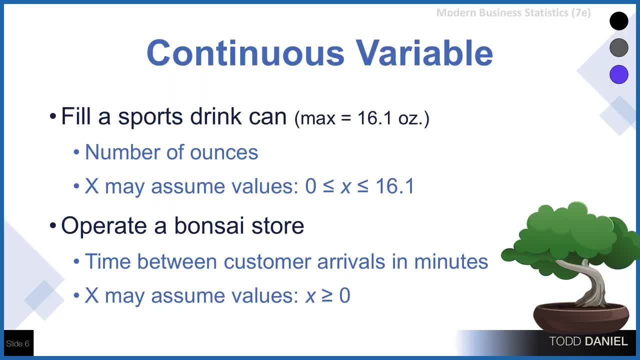 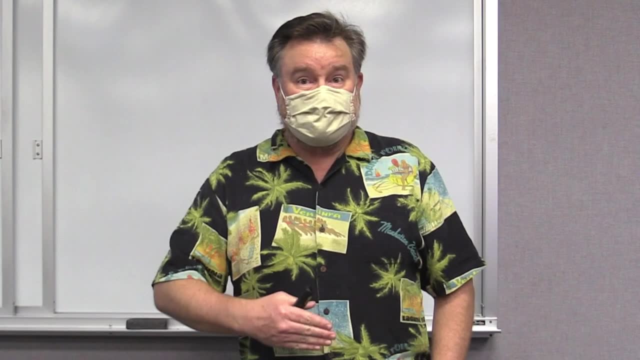 It should be some kind of value in between that range. Or you're operating a store. I just picked a bonsai store for no reason other than I happen to have a picture of a bonsai tree easily available. Any kind of store, any kind of business. How many minutes between each customer's? 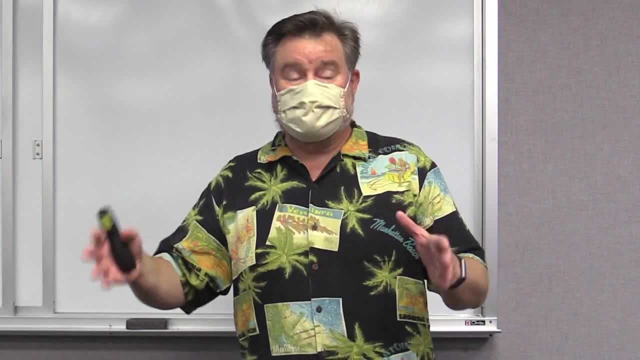 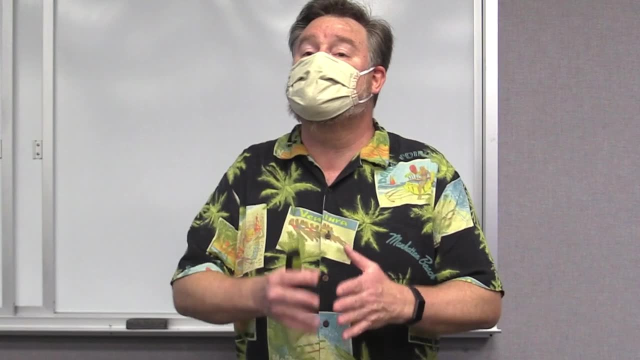 arrival. There may be stretches of time when no one shows up And there may be other times when two or three or four customers show up at almost the same time. There's very little time in between. So how many ounces of fluid are in the can Theoretically could range from 0 all the way to 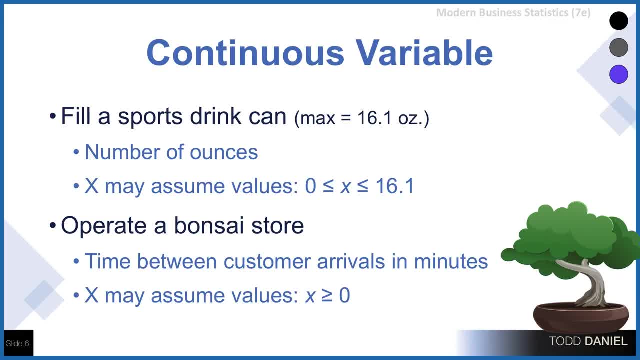 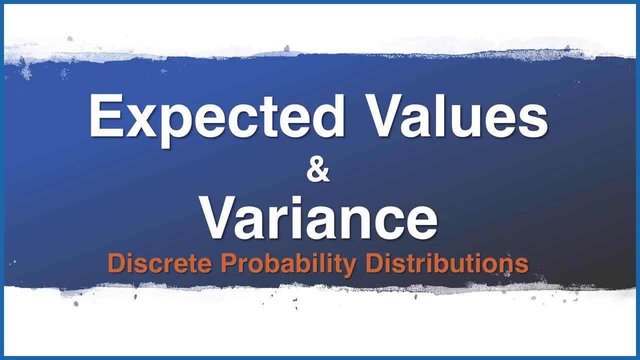 16.1 or she's able to Prison This value can assume any value greater than 0.. 0 being our lower bound but an infinite upper bound. We'll talk about this type of distribution next time. Right now, we're going to talk about discrete probability distributions and start with expected values. 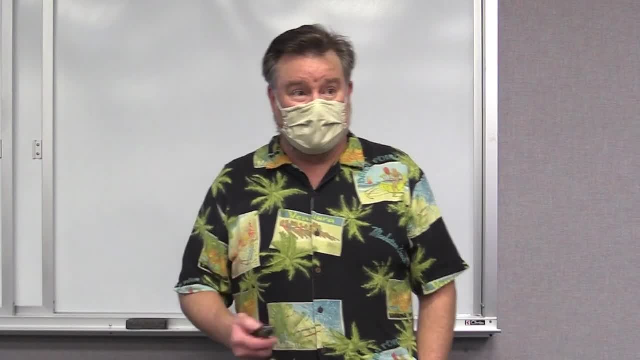 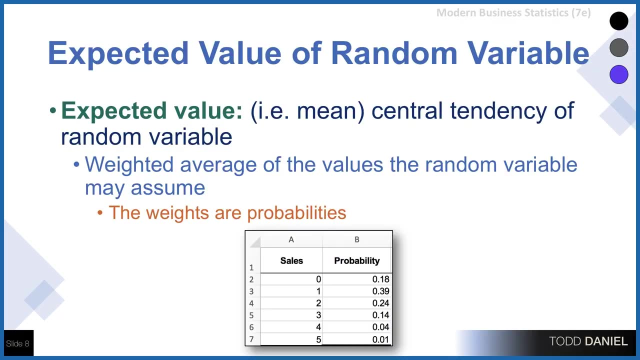 and variance. An expected value, when we talk about probability distribution, is the mean And it really is a weighted mean. So an expected value is a measure of central tendency for a random variable. In this example I have sales and the probability of making a sale of 0,, 1,, 2, or 3 sales. 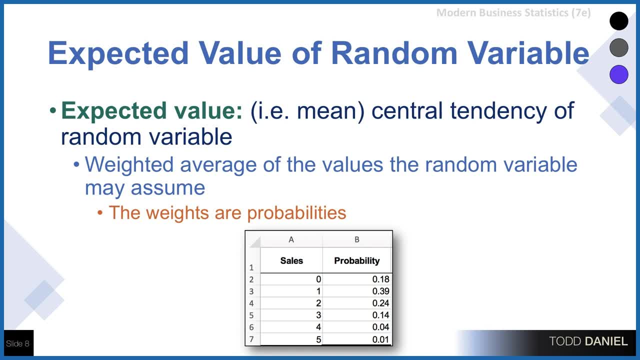 The weights are the probabilities. So if we were going to calculate a mean, we would multiply the sales number by the probability and we would use that for calculating our mean. And we're going to get a chance to do that using Excel here a little later. 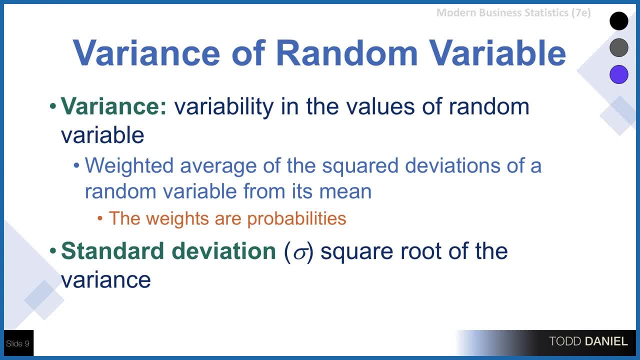 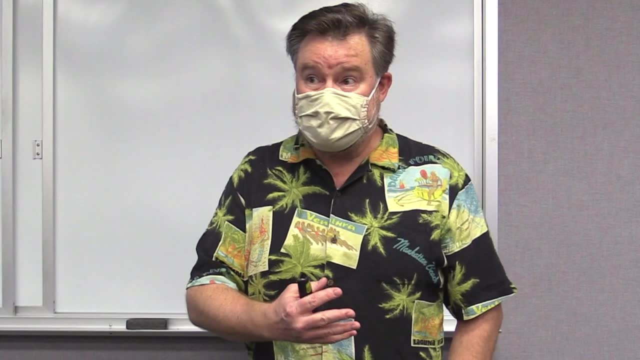 The variance and the standard deviation. Variance is a measure of variability for a random variable. It is still a weighted average of the squared deviations. Remember that a deviation score is x minus the mean. So once we've calculated a mean, we can subtract the mean from each of the sales numbers. 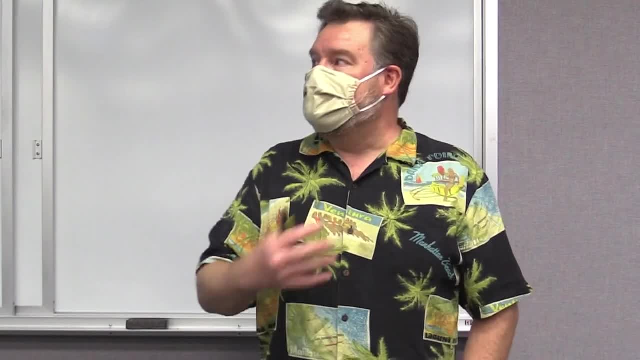 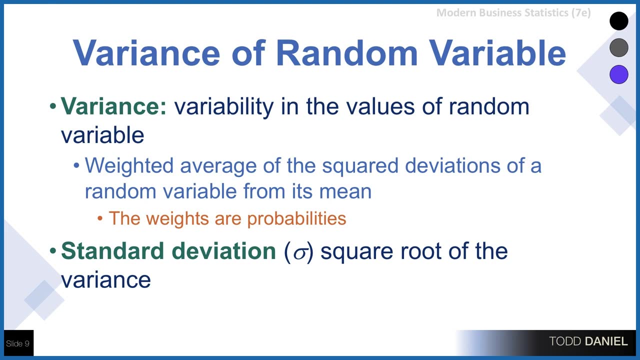 square those values, add them up, divide by the total number And that's going to give us variance. The standard deviation, therefore, is the square root of the variance, in the same manner as we had calculated square root using any other distribution of numbers. 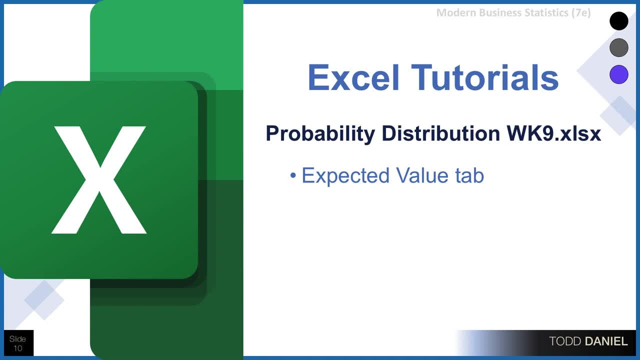 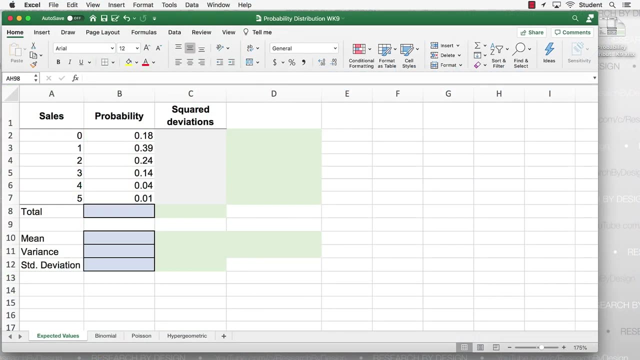 This week I've created an Excel tutorial that is titled Probability Distribution- Week 9.. And there are multiple tabs across the bottom of this Excel tutorial. We're going to start with the expected value. It's going to look like this, with just the blanks. 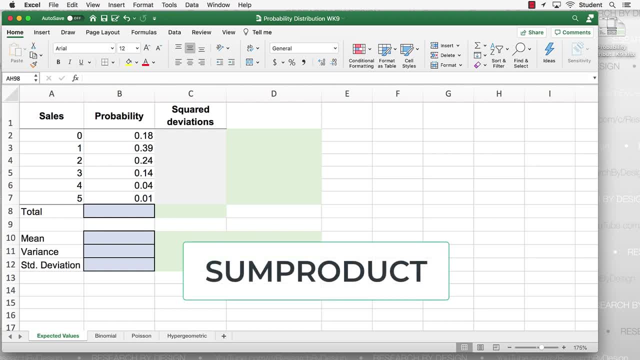 We will be learning the sum product formula in order to use these techniques. The sum product means multiply one value times another value and then add up the totals. So here's how we would do this. The first thing that we need to make sure is that all of our probabilities add up to 1.. 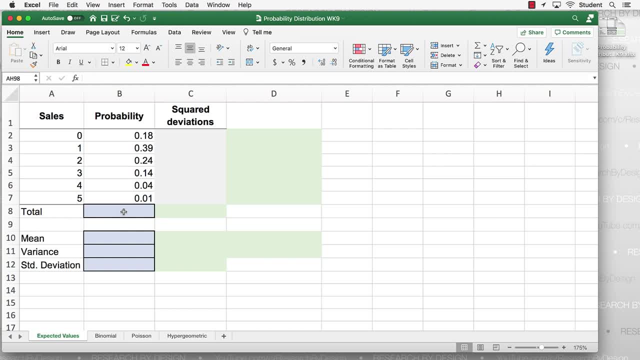 So we could check that By going to cell B8, and we would type equal sign sum B2 to B7. And sure enough, our probabilities add up to 1.. So we're good for this next part. Now we're going to create the mean. 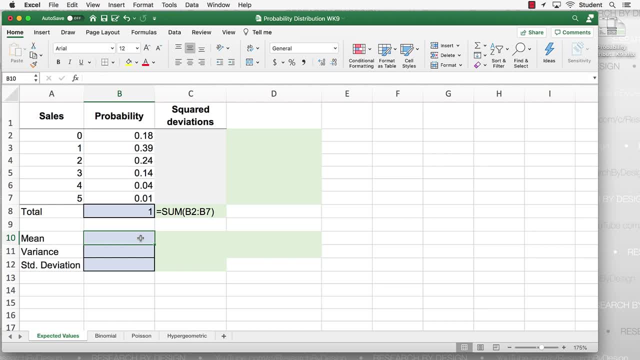 In cell B10, we're going to use the sum product formula, So it's equal sign: sum product- open parenthesis. Our first array would be A2 to A7. And our second array is B2 to B7. This gives us an average of 1.5.. 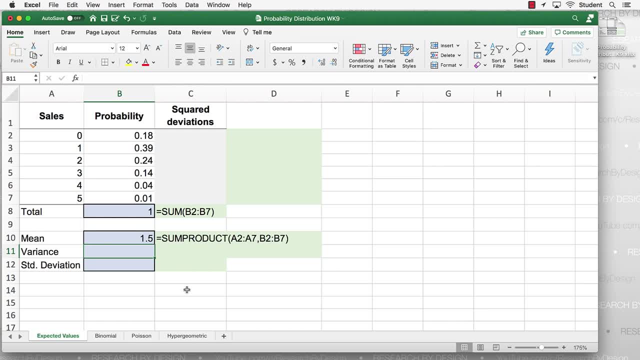 And that was calculated by multiplying the sales figure times the probability That product is then added up or summed, giving us a total of 1.5.. So that means that we expect that the average sales figure is going to be 1.5.. 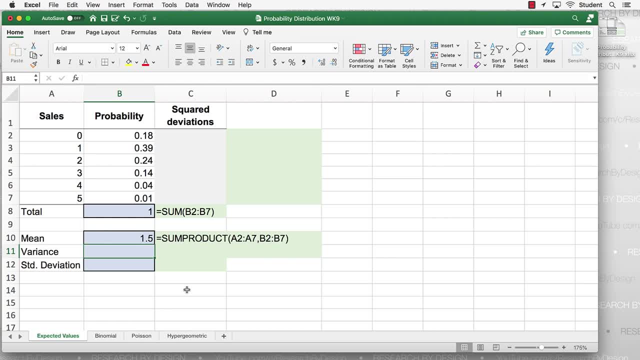 And the average sales will be 1.5 sales per day. Now we can calculate the squared deviations and again use the sum product. So the squared deviations X minus the mean. Our formula therefore will be equal. sign open parenthesis: A2 minus B10, which is our mean. 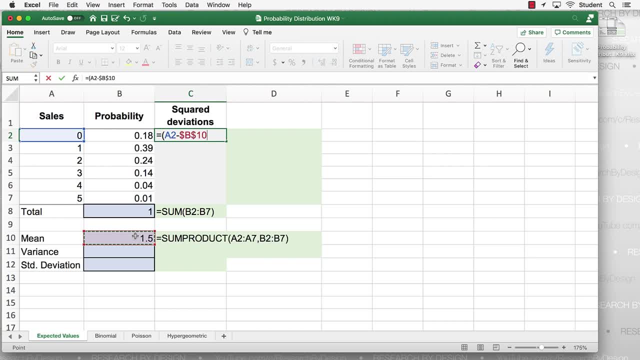 And be sure to anchor or make this an absolute reference by using either command T on your Mac or F4 on your PC. That's the dollar signs around the B10.. Close parenthesis. and then we want to multiply that by itself or square it. 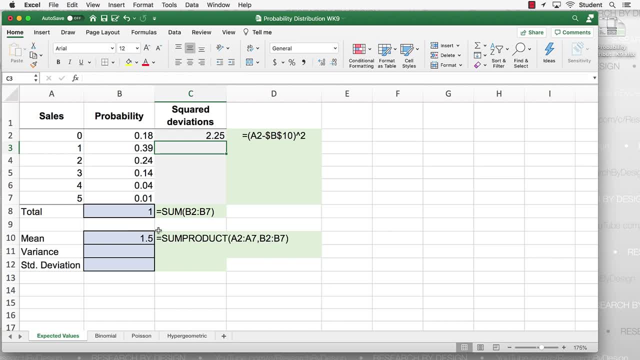 So caret. 2. Hit return. Now we have a squared deviation for our first set of sales of 2.25.. And we can drag our formula down to C7 to calculate these squared deviations. Now we're going to use the sum product on the squared deviations to get the variance. 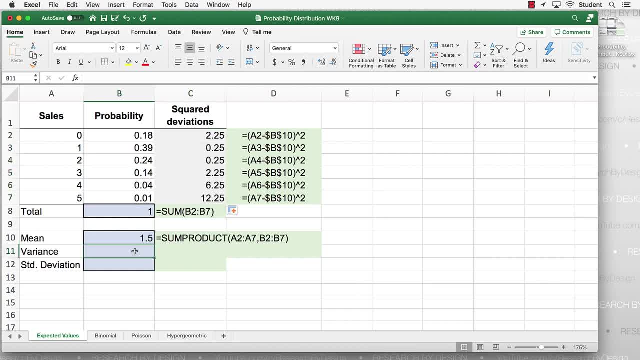 So in sales, So in cell B11, type sum, product C2 to C7, comma B2 to B7.. And this gives us our variance. Remember, variance is a squared value, so we want to unsquare that. take the square. 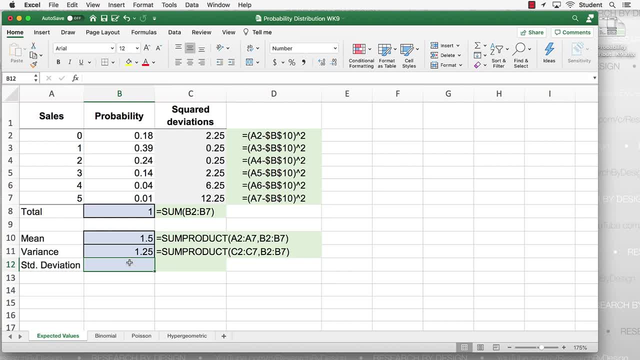 root of it. So now in cell B12, square root of B11 gives us our standard deviation And we would interpret this by saying: the variance of the daily sales is 1.25.. Standard deviation of daily sales is 1.118.. 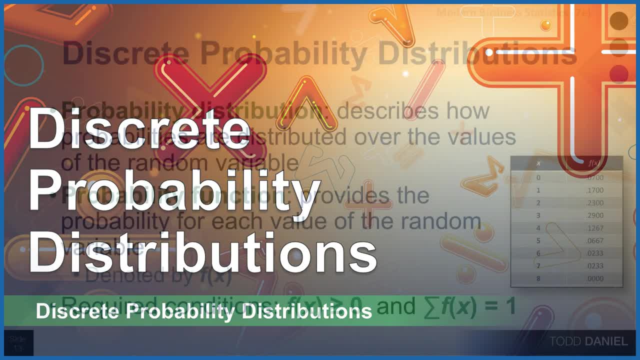 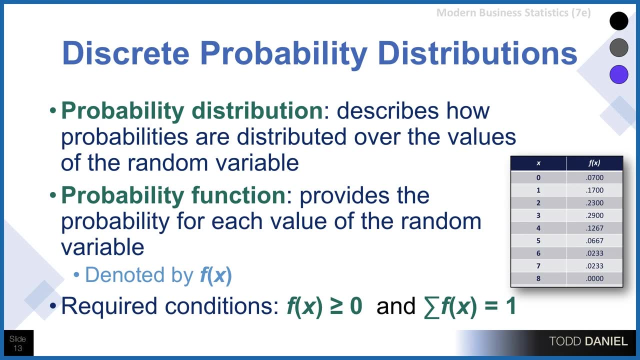 So next we're going to talk about these discrete probability distributions. A probability distribution describes how the probabilities are distributed over the values of the random variable. So, if you look at this example, Okay, Okay. So the probability distribution is going to range from zero to eight. 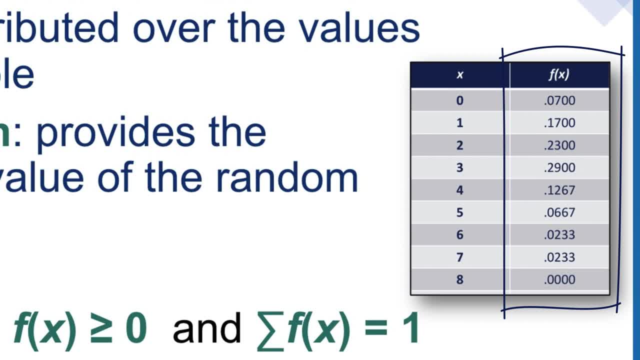 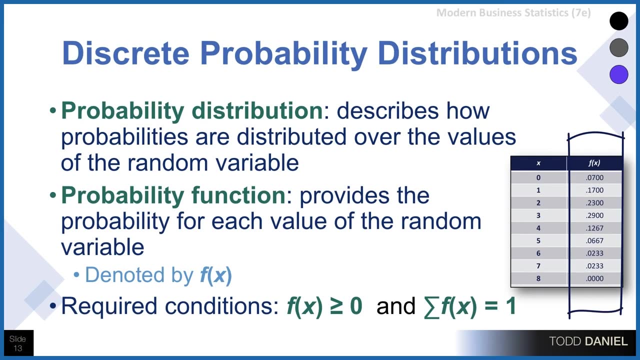 A probability function is the probability of each value of the random variable which is notated by the fx. There are two conditions that we need to meet to use this. The first is that these probabilities must be greater than or equal to zero. So you notice, there is a zero probability for the x value of eight, but there are no. 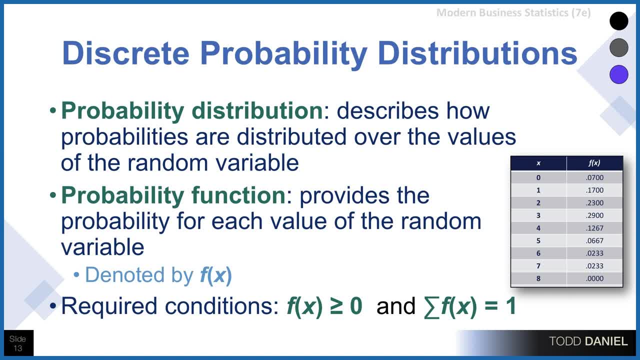 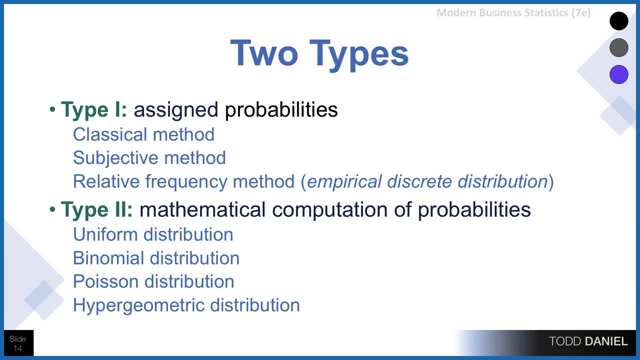 negative values. And the second required condition is that when we add up all of these probabilities, they must add up to one. Now there are two ways that we could assign probabilities. We could use the classical method, the subjective method or the relative frequency method. 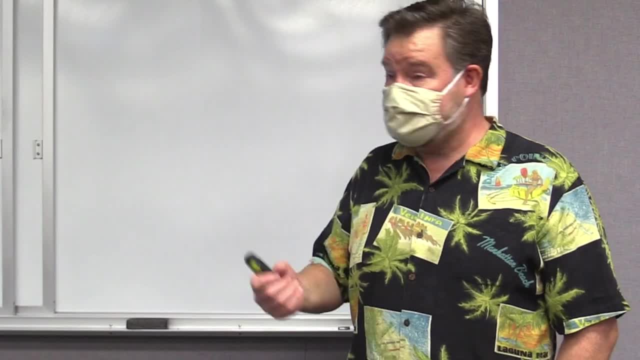 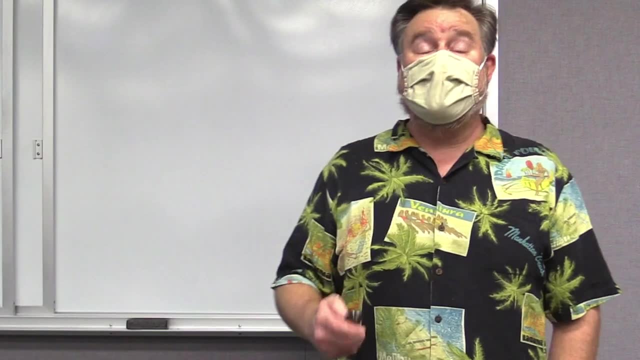 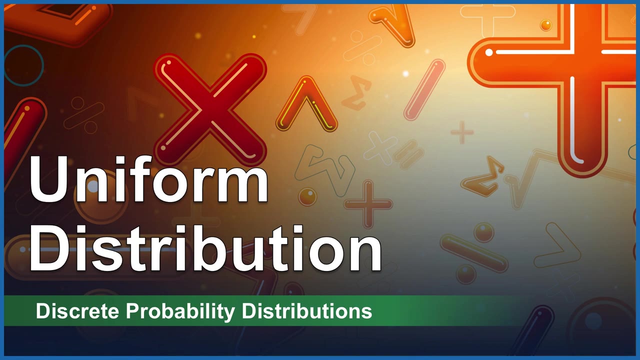 Or we could mathematically define, using either the uniform distribution, binomial distribution, Poisson distribution or hypogeometric distribution, And that is what we're going to do, Okay. So what are we going to do now? We're going to start with this uniform distribution, which will be the first discrete probability. 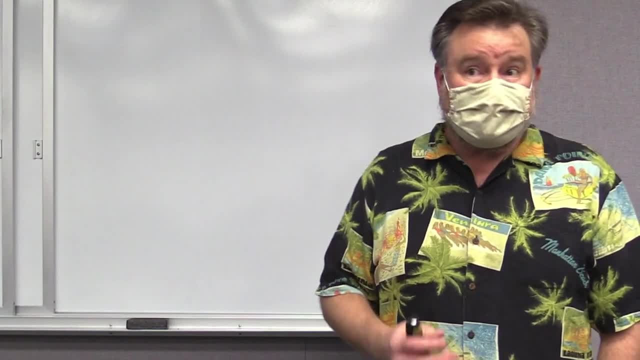 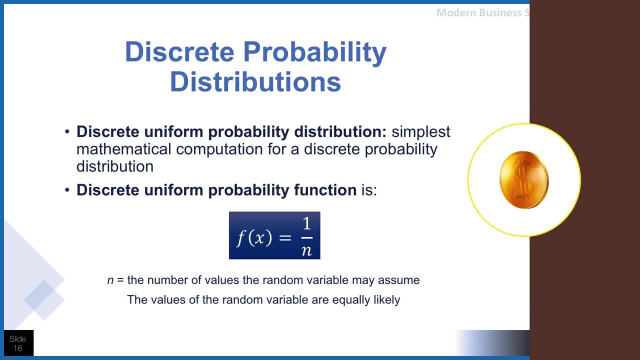 distribution that we'll learn about And it is the simplest. This best example for flipping a coin or rolling a die: The discrete uniform probability distribution. The function is one over n. Flipping a coin. Coin has two sides. The function or the probability would be one over two. 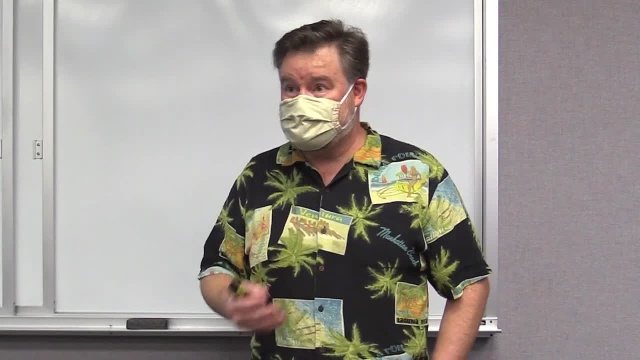 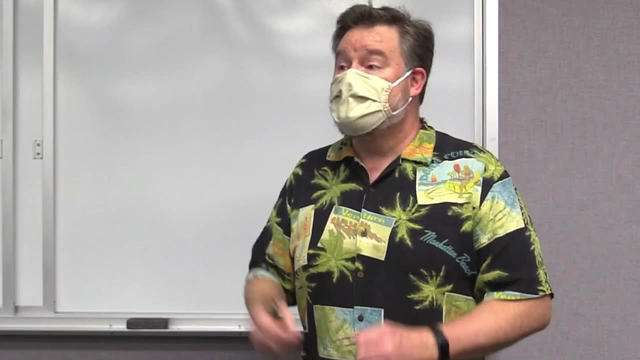 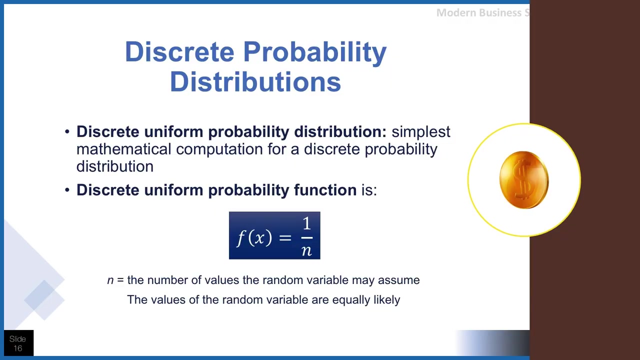 Or 0.5.. There is a 0.5 probability of getting heads, 0.5 probability for getting tails. Same logic for rolling a single die. It has six sides. You roll that, die the options. the probability of any side coming up is one over six. 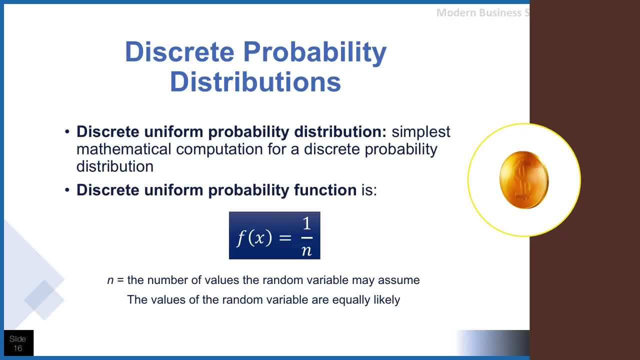 So n is the number of values. the random variable may assume Two sides to the coin, six sides to the die, 52 cards in a deck, And the values of the random variable should be equally large. Likely The coin is fair. 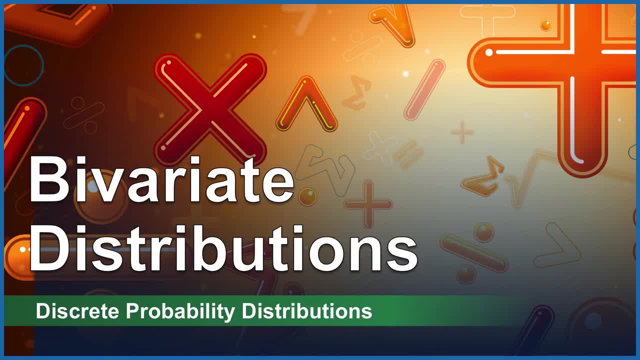 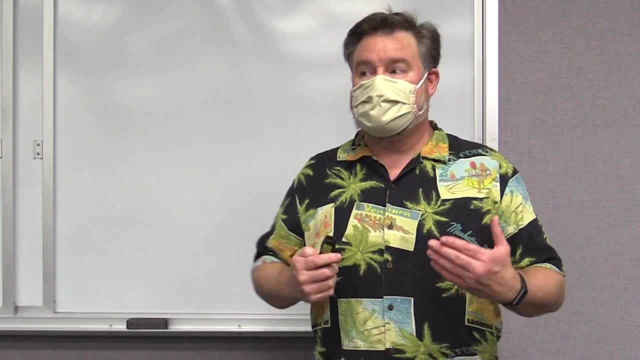 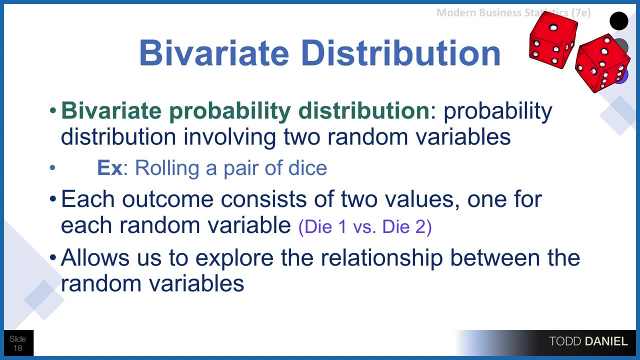 The die is fair, The cards have been shuffled thoroughly. The second distribution is a bivariate distribution. Bivariate means two variables. Bivariate probability distribution is the probability distribution involving two random variables. Now we're not just rolling one die, we're rolling two at a time. 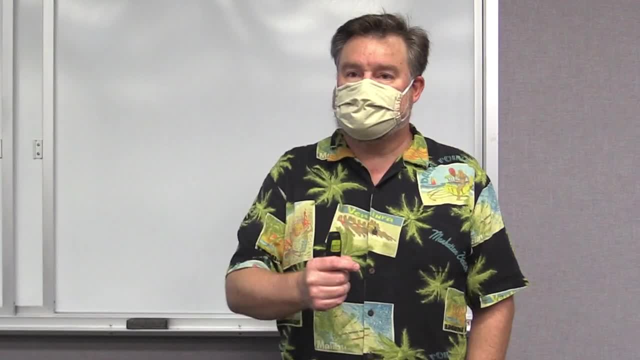 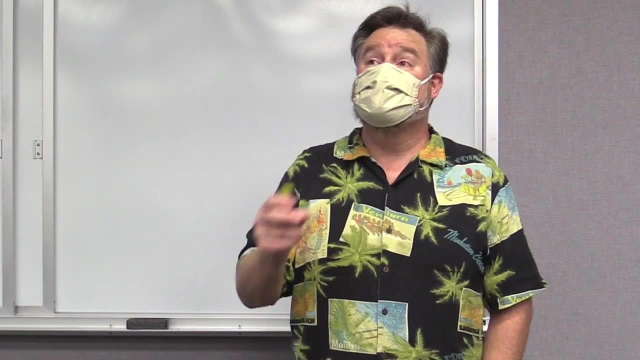 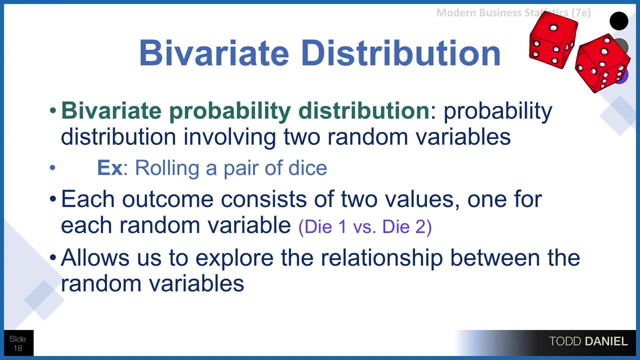 And each die could have an outcome of one to six. We would consider the outcome for die number one and then the probability for die number two. So each outcome consists of two values. that's what makes it bivariate. We're considering both of those die together. 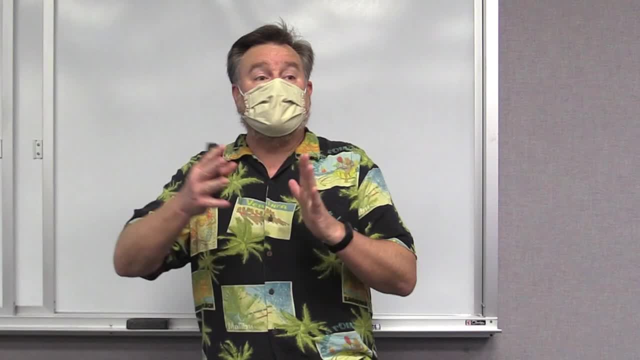 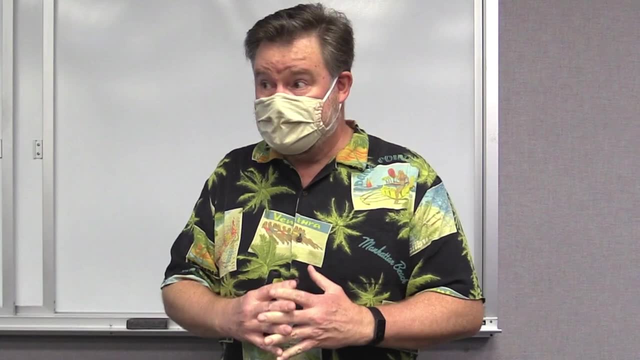 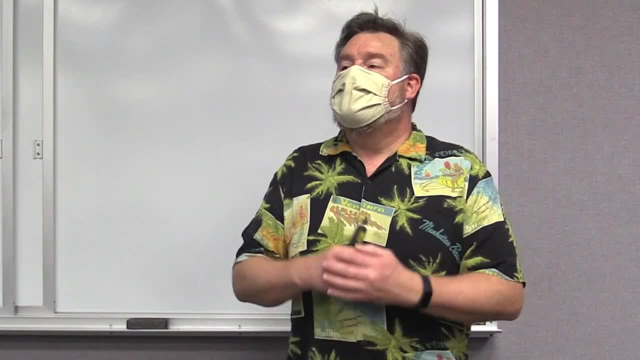 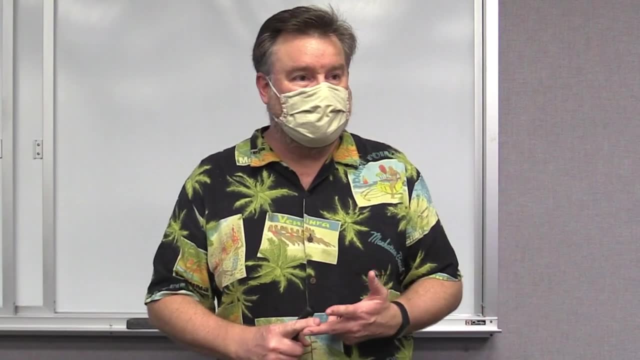 What would be the largest number? A six on each die. total of 12.. But what value would have the most ways of getting to this value? The value for seven we could get to is a six and a one, a five and a two, a four and a. 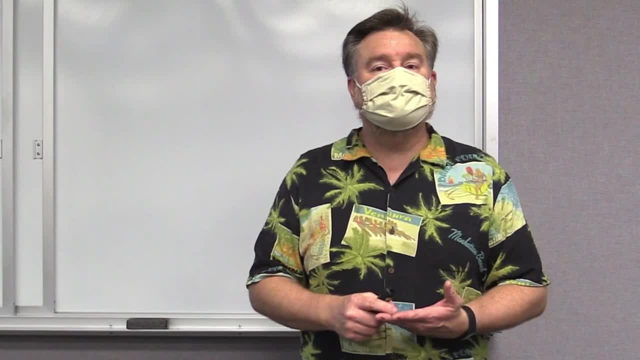 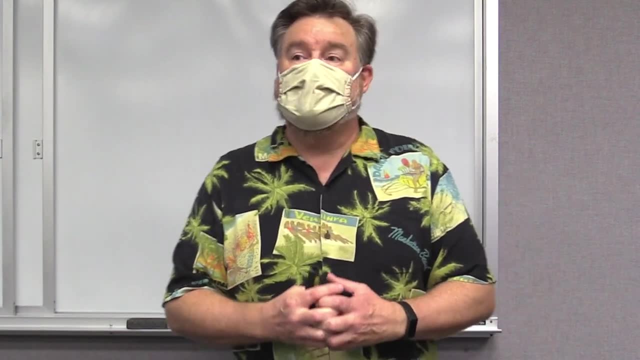 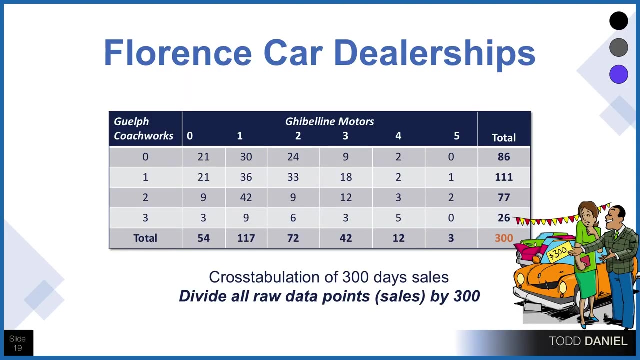 three, a three and a four, a two and a five. So there are many ways to get to seven. So we would expect to see seven, seven occurring more commonly with this bivariate distribution than we would expect to see rolls of one or of twelve. So now we can examine the relationship between these random variables. 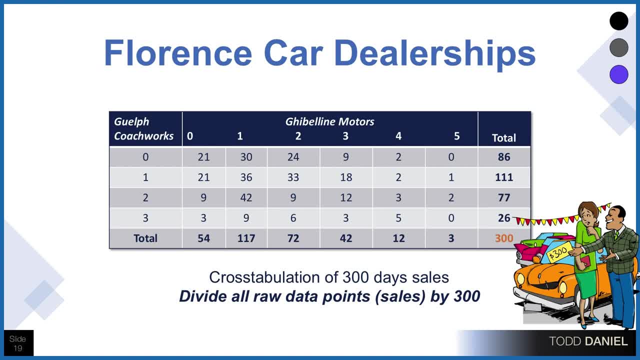 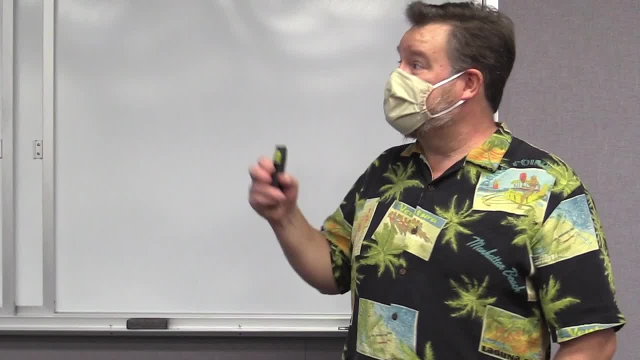 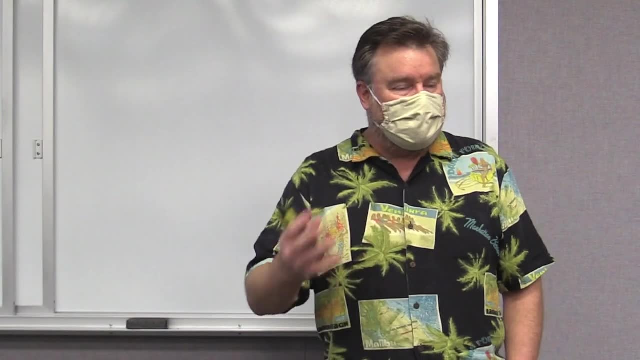 For this I'll use the example of a car dealership, the Florence car dealerships. There's two in town. We have Ghibelline Motors and the Guelph Coachworks. The Ghibelline Motors is a little larger. They sell more cars on any given day or week, and so their range of cars they would sell. 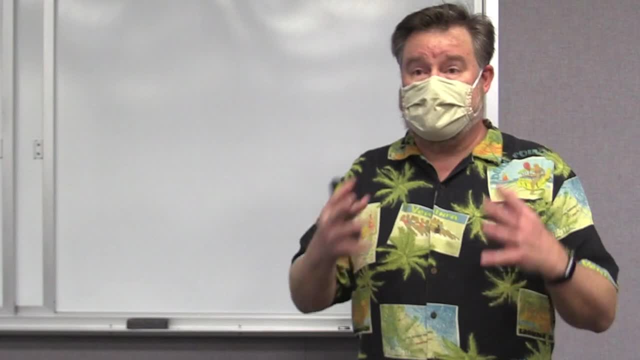 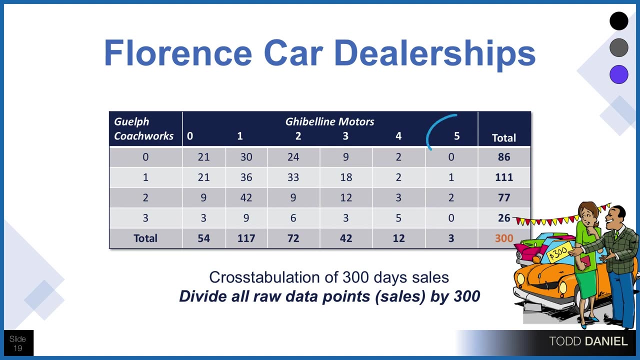 runs from zero to five. This is based on observing how many cars are sold each day. for 300 days, The most number of cars that they sold on any day was five. For the Guelph Coachworks, the greatest number of cars that they sold on any given day was three. So we have two variables: the sales for each. 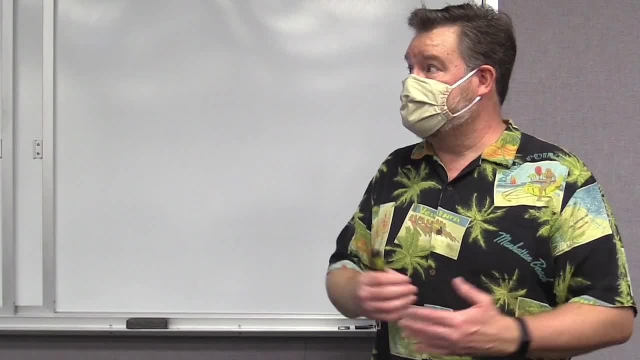 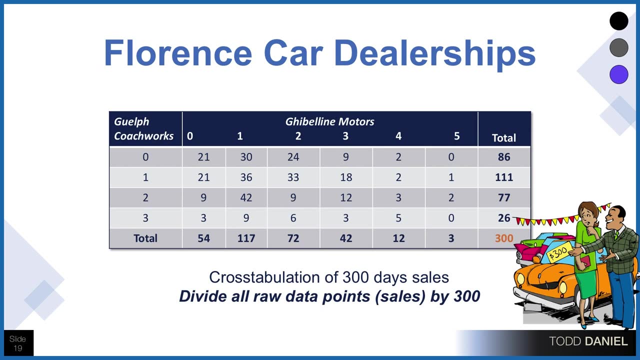 of the dealerships giving us a bivariate distribution. So you can see, what we've started with are just some raw numbers. The number of days in which both dealerships sold zero cars was 21.. The number of days in which Ghibelline Motors sold one and Guelph sold zero was 30.. The number of days when 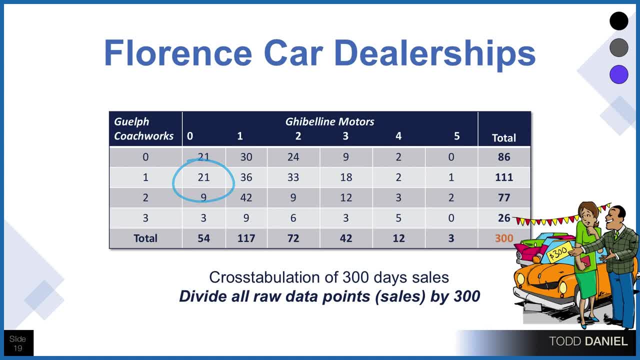 Ghibelline sold zero and Guelph sold one was 21.. The number of days in which they both sold three was three, And all of these values added together add up to 300.. What we would then do is divide each one of. 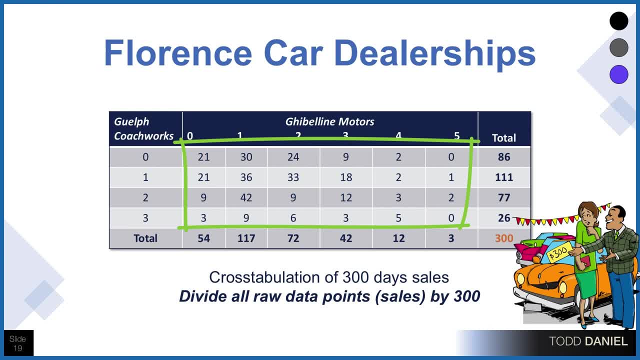 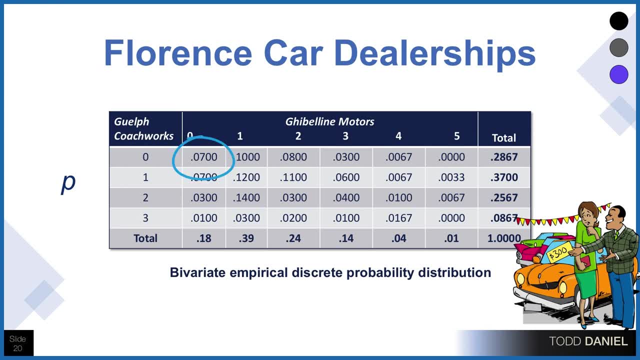 these sales numbers by 300, and that's where we're going to get our probabilities. What is the probability that both sold? zero, It's a 0.07.. The probability that both sold three would be 0.01.. There's one other thing that we would want to get in order to create our frequency. 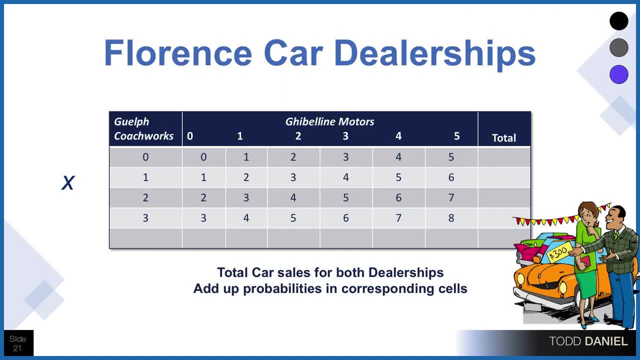 the table out of this And that would be the number of ways that we could get to sales of zero or one or two. So if you look on the diagonals you see that there are many ways that we could get to. 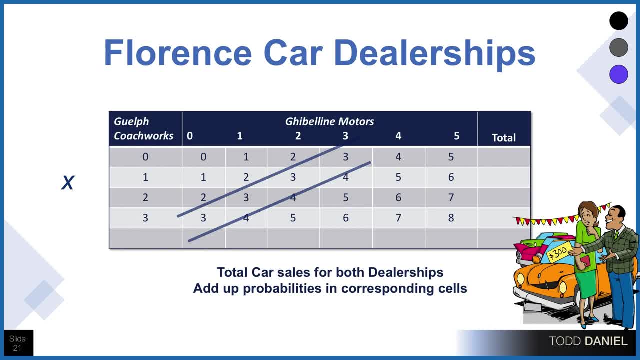 three sales. One is the first dealership sells three, the second sells zero, or one sells two and the other sells one, or the opposite of that: one and two, or zero and three. So there are four options for getting to three sales, And each one of those has a probability associated with it. 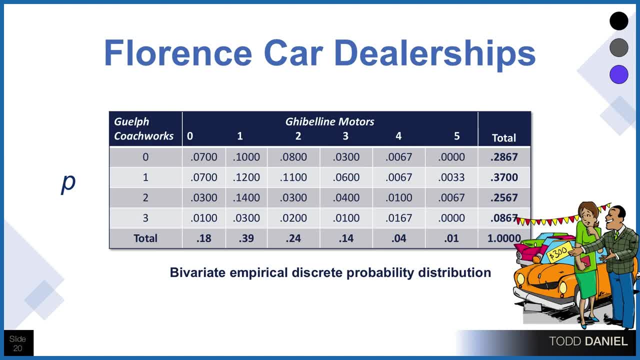 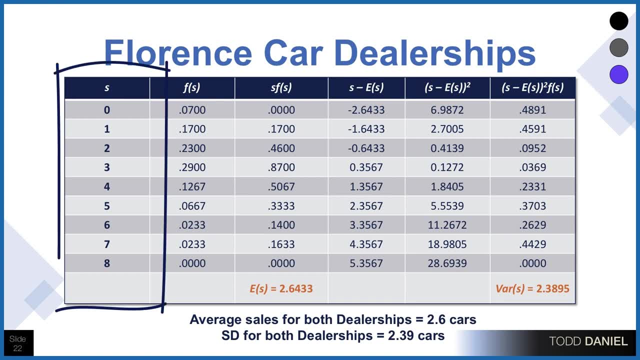 We would add up all those associated probabilities and then we could put those into a table that looks like this: Our column, which we're using S to stand for success or sales, ranges from zero to eight. The sum of all the probabilities to get to any of these sales figures are added up in the 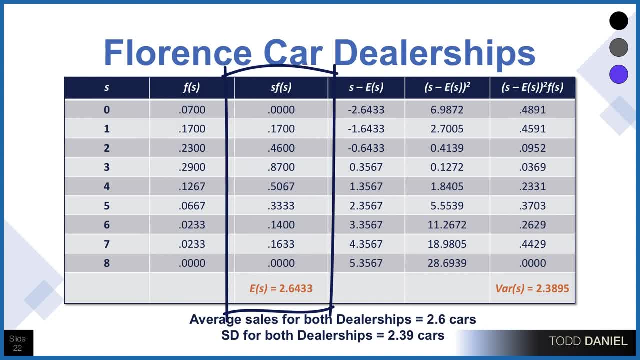 second column, And then we can multiply the sales figure by the probability to give us the values that we need to add up, divide by eight and get to our sales figure. So it's a 2.6433.. We would say that the average sales for both dealerships is 2.6 cars, And then we could create our deviation. 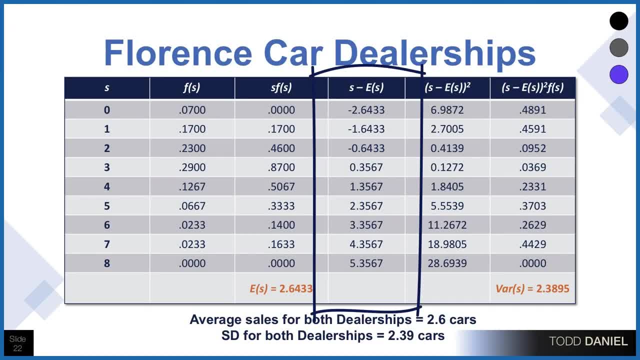 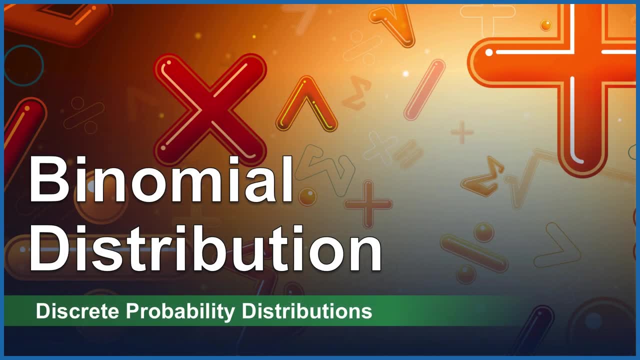 scores By subtracting the sales figure from the mean, and then we would square that value, add it up, divide by eight and it gives us our variability. Take the square root of that would be the standard deviation And a binomial distribution different than a bivariate distribution. Binomial is: 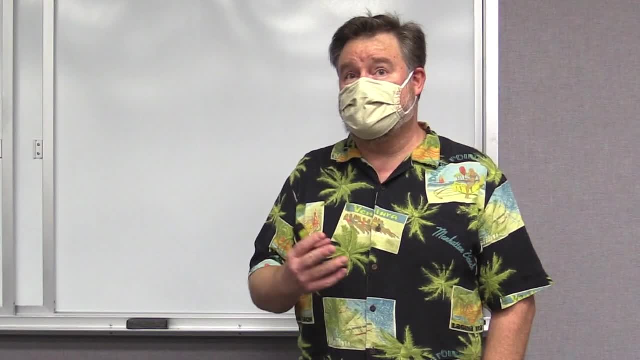 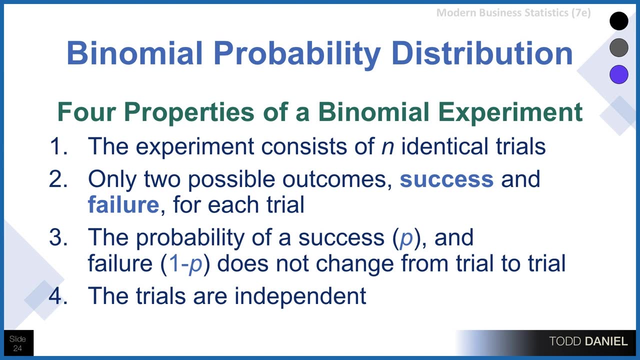 referring to the number of outcomes. So we use a binomial distribution when there are only two outcomes available. Four properties of the binomial distribution are the number of outcomes and it's the number of times they flip the coin. And, for example, if you do a binomial experiment, 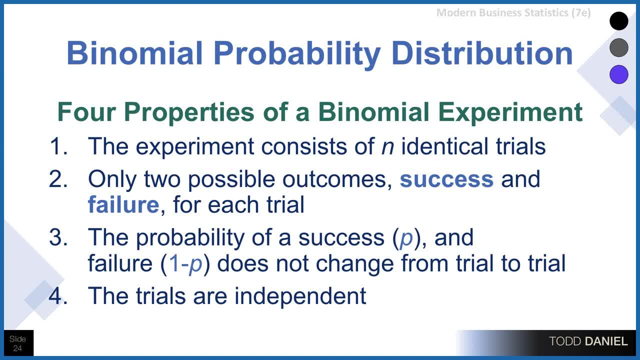 the experiment consists of n number of identical trials. Think of flipping the coin. You flip the coin. it's identical to the next flip of the coin. There are only two possible outcomes, which we would call success or failure. Let's say we're keeping track of the number of heads that were 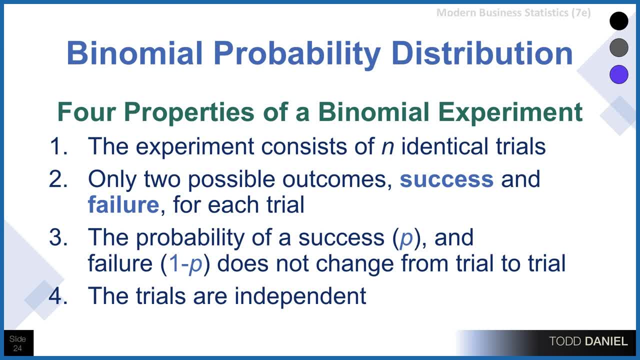 flipped with each flip of the coin. Number three: the probability of a success and the probability of a failure do not change from trial to trial, They're independent. So that, defending those gains, and then the second step, we can say that there are actually two ways of finding out how the sales figure 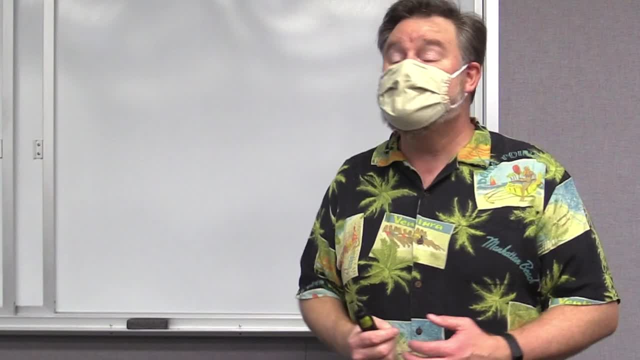 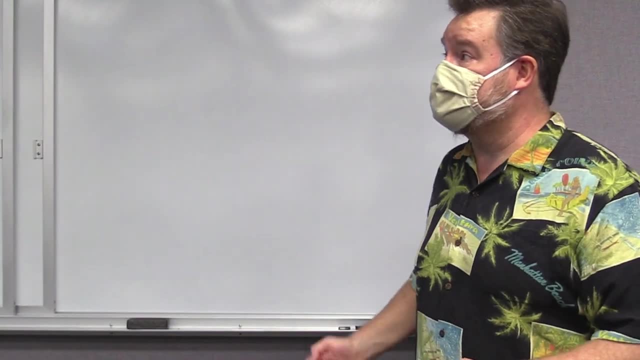 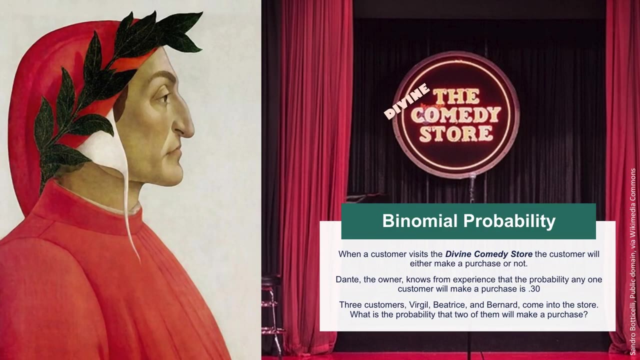 So that the flipping of the coin when it comes up heads on this flip has no effect on what the coin will flip in the next trial, being independent of one another. So if we have satisfied all of those, let's use this example. When a customer visits the Divine Comedy store, the customer will either make a purchase or not. 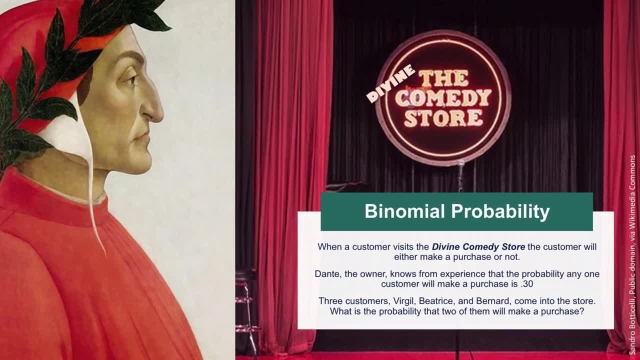 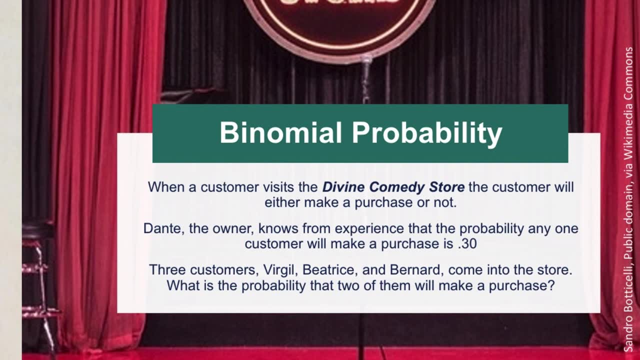 And you could apply this to any business. The Dante, the owner, knows from experience that the probability of any one customer making a purchase is 0.30.. This is from historical sales figures. Three customers- Virgil, Beatrice and Bernard- come into the store. 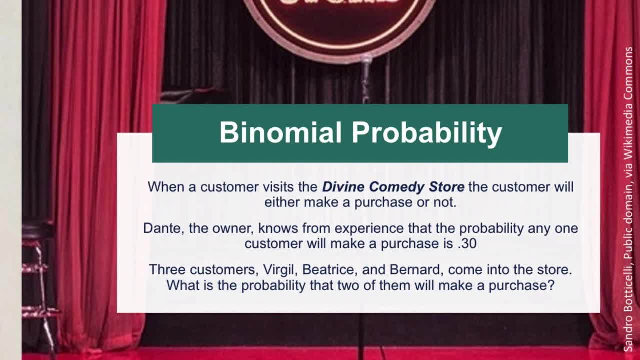 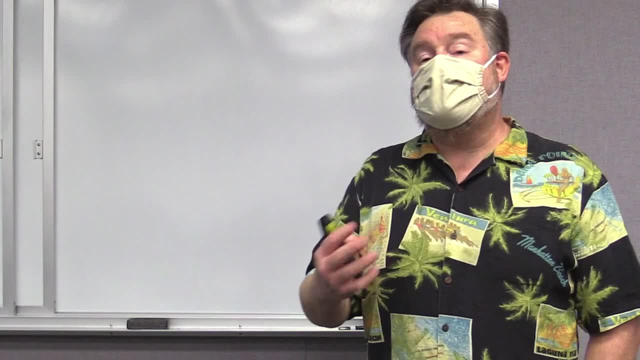 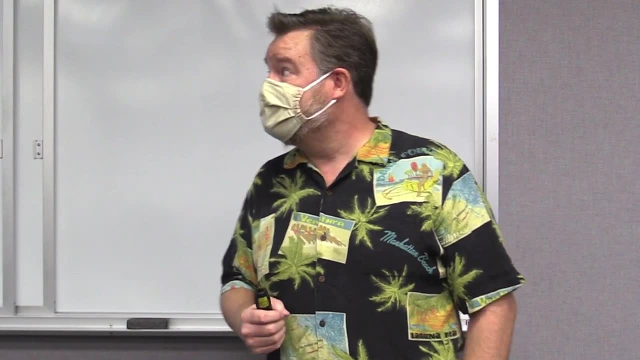 What is the probability that two of them will make a purchase? What we would first need to consider are the facts that we have available to us. We know the probability of any one person making a purchase is 0.30.. We know there are three customers who have entered the store and we're interested in the probability of two of them making a purchase. 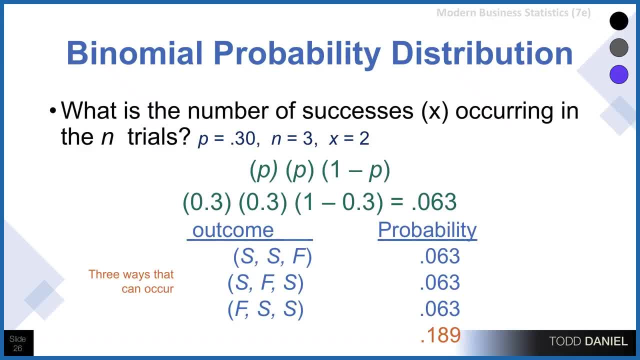 Now we could start this very simply by just taking the first probability, multiplying it by the second, and then the third person doesn't make a purchase. So that's 1 minus the probability, which, of course, is 0.3.. So it's 0.3 times 0.3 times 1 minus 0.3, which computes to 0.07.. 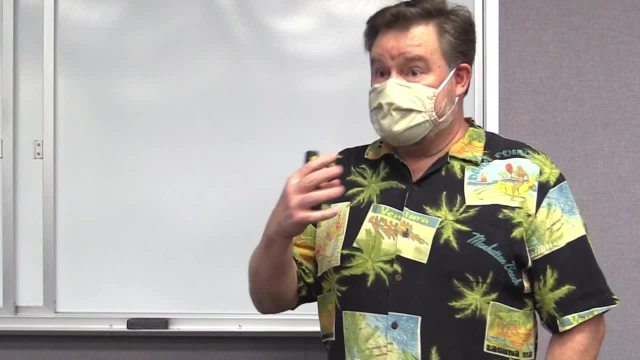 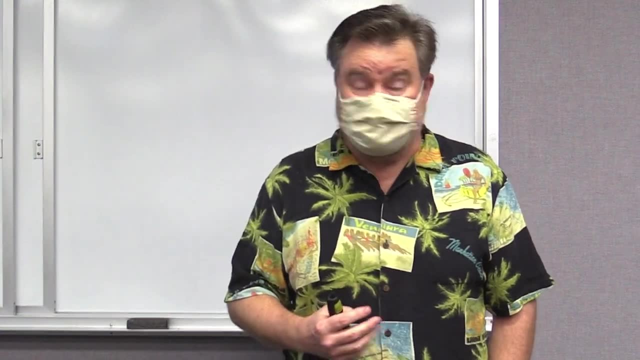 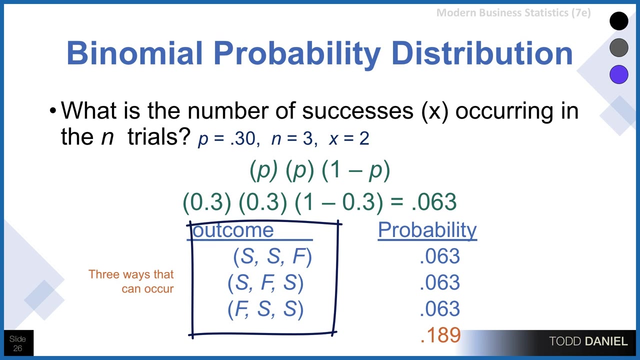 That is the probability for just two of them making a purchase, But remember, there are three different ways that we could arrive at that outcome. The first two people make the purchase, the first and the third, or the second and the third, each of which has a probability of 0.063.. 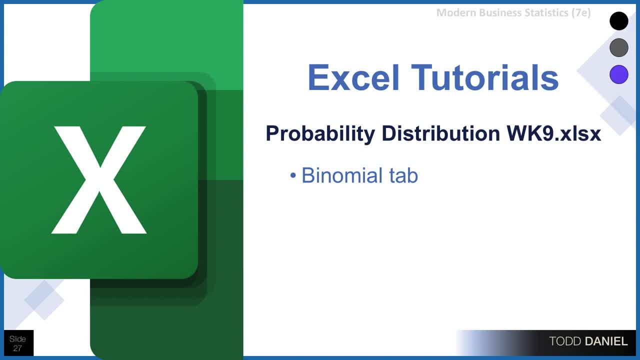 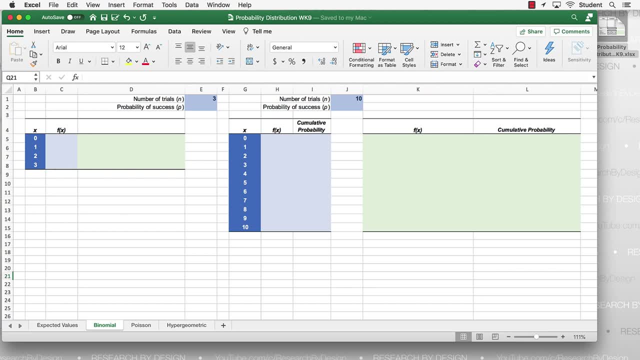 I can also use the Excel tutorial on the Binomial tab to illustrate this outcome. I'm going to go ahead and do that. I'm going to do this twice. In one example, we're going to have three people enter and we'll use our probability of success and figure out binomial probabilities. 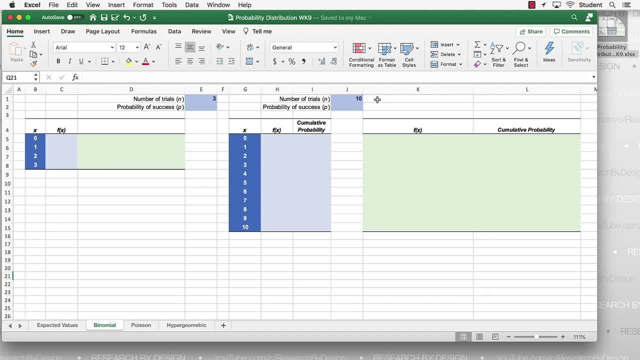 And in the second example, 10 people, 10 customers and the probability of success will stay at a 0.3.. And we'll also use cumulative probability for this example. So, number one, the number of trials or customers, is 3, and the probability is 0.3. 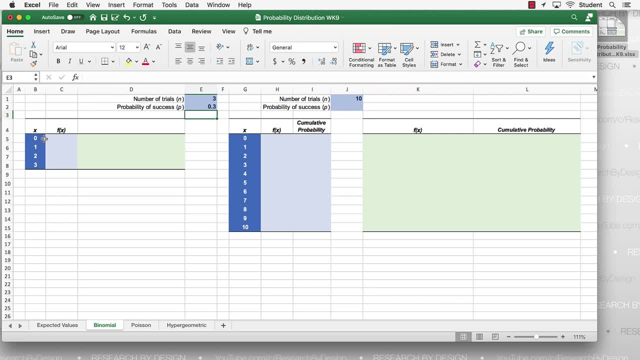 I've created a table with 0,, 1,, 2, and 3 as my x values And my probabilities I would get from: I would go to C5, and, using the binomial distribution, I would type equal sign. BINOMDIST for binomial distribution. 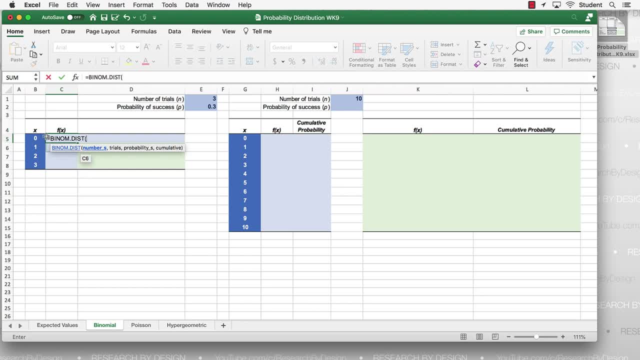 So I want to begin by referencing the x value, in this case B5, comma, and then E1.. E1,, which is the number of trials- I want to make that an absolute reference with the dollar signs around it. E2,, which is the probability of success. 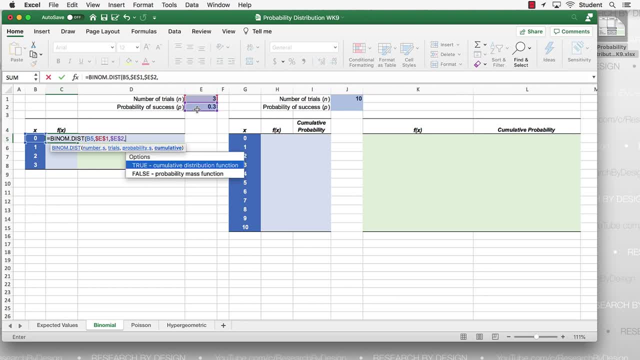 Again, anchoring it, dollar signs around it And then false, which is going to just give me the probability for that outcome. Close parentheses: and I've created a function value: It's a 0.343.. Great, I can now drag that function down. 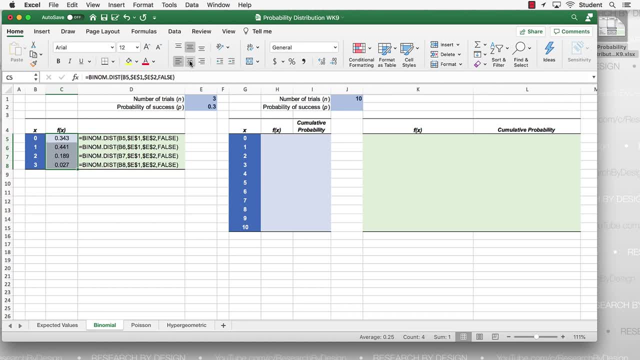 And I've completed. I've completed my table. So what is the probability for 0? It is a 0.343.. Or the probability for 3 is a 0.027.. What if there are 10 customers? Well, if the probability of any particular person making a purchase is still the 0.3,. 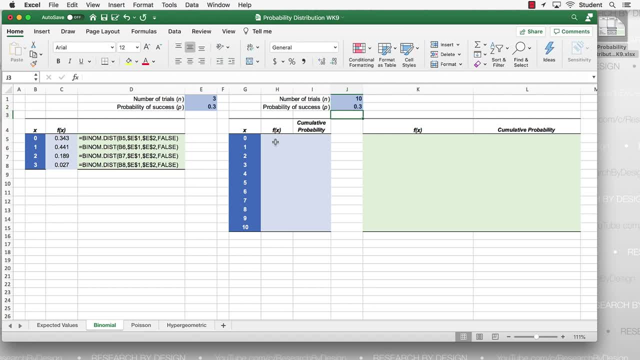 I can fill in my probability table ranging from 0 to 10.. Starting in cell H5, I would type: equal sign Binomial distribution, open parentheses- G5, which is the first sales number, J1,. the number of trials: J2,. the probability of success, both of those as absolute references, and. 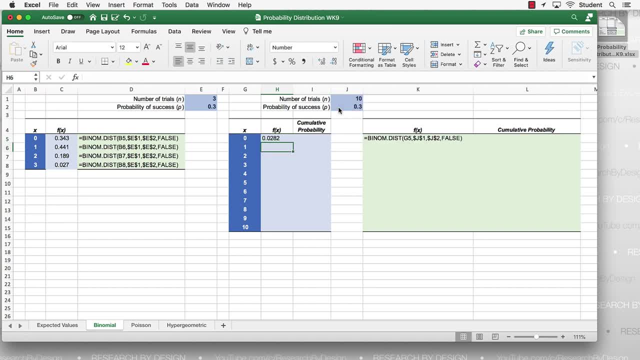 false. Close parentheses now drag that formula down. I've filled in my first column. The false option gives me just the probability, But sometimes I want to get the answer. I want to get the cumulative probability adding up all of the scores up to that point. 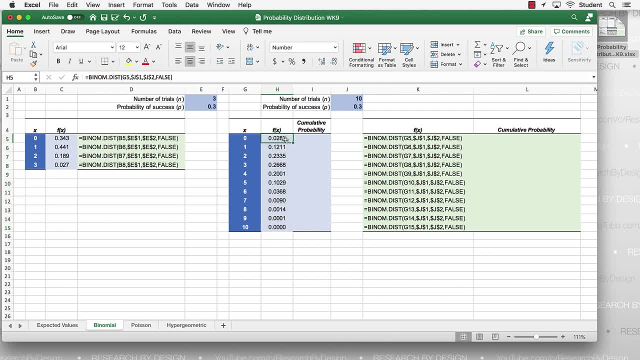 To do that. what I would start by doing is I would go to cell H5 and just drag that 1 to the right and create a duplicate. except I'm going to have to clean this up a little bit, So I'm still using the binomial distribution. 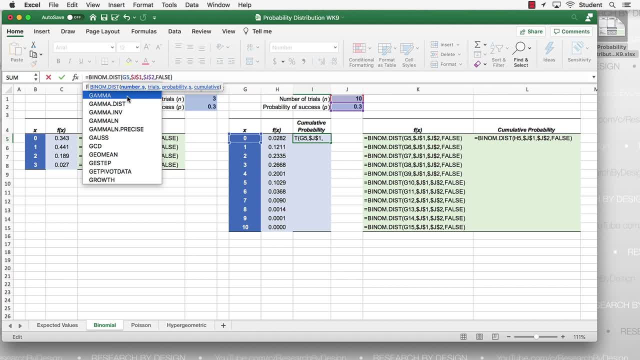 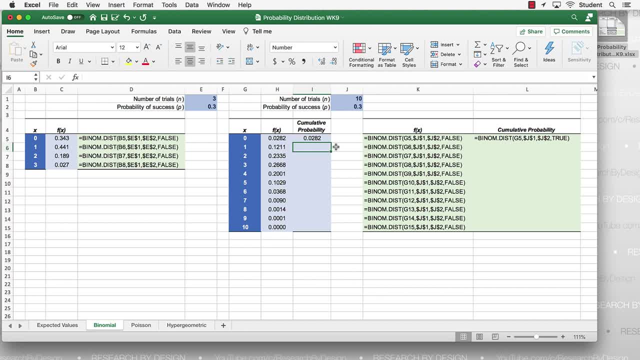 And I'm going to go to cell H5.. And I'm going to go to cell H5.. Having done that, I can drag this option down And I've filled in my cumulative probability table. So what is the probability, given 10 customers, that at least three, or let's say three or 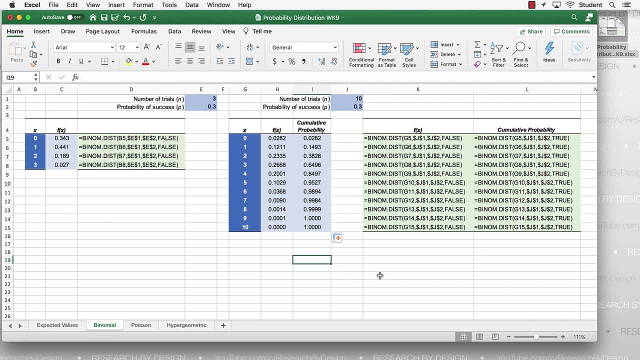 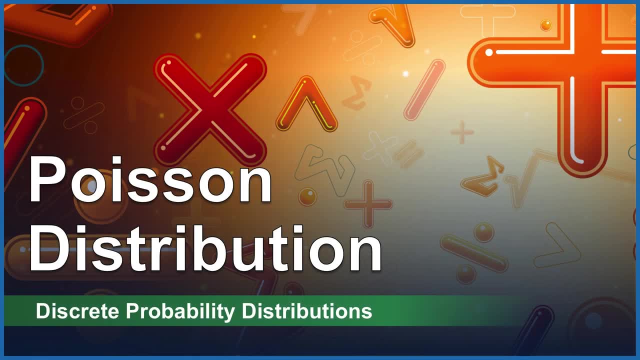 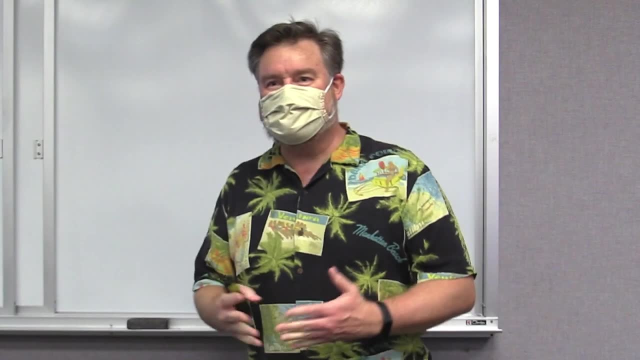 fewer will make a purchase of a 0.646 or fewer, 0.98.. So that brings us to the Poisson distribution. Poisson in French means fish. You may remember one of my favorite scenes from The Little Mermaid, the Disney classic. 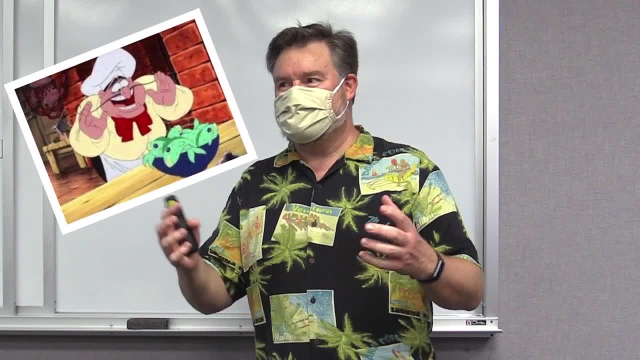 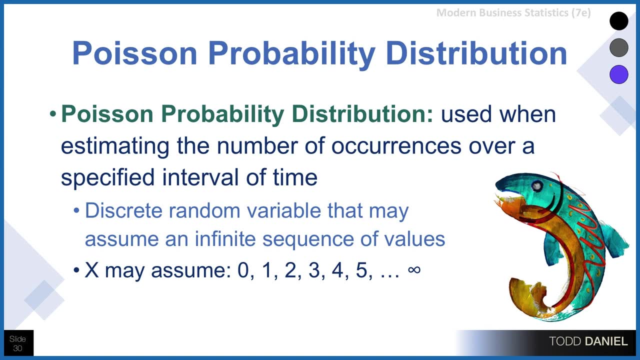 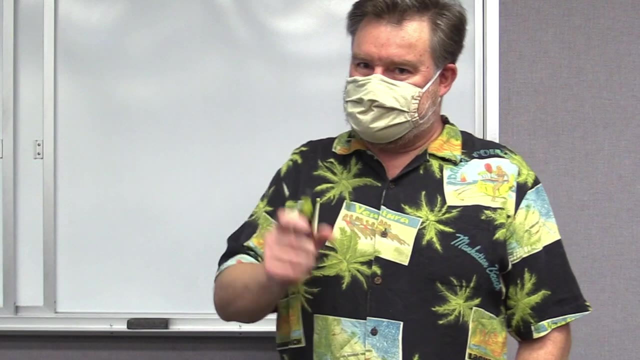 was the French cook singing about le poisson, le poisson singing about cooking up fish. Poisson distribution is used when estimating the number of occurrences over a specified interval of time, And it could be over any specified interval, but we just have to make sure that that interval 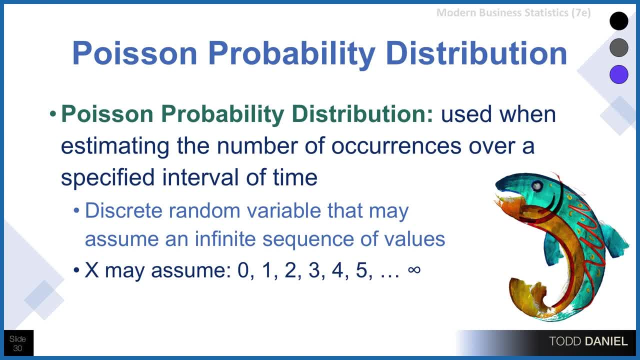 is accurate. Okay, Okay, Okay, Okay. So this is a Poisson variable, It's called the Poisson distribution And it's a mean of negative to, I guess, negative or less threatening, always consistent. It is a discrete, random variable that may assume an infinite sequence of values. 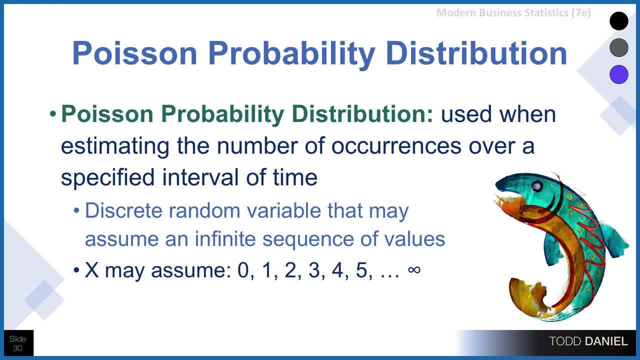 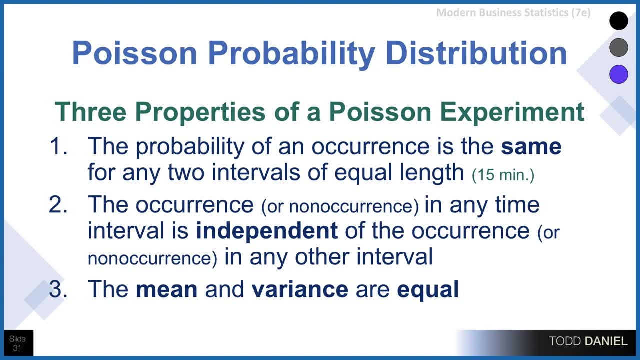 So they're going to be whole numbers starting from zero, one, two, three, four, five, all the way up to infinity. Three properties of a Poisson experiment. Number one: the probability of the occurrence will be the same for any two intervals of. 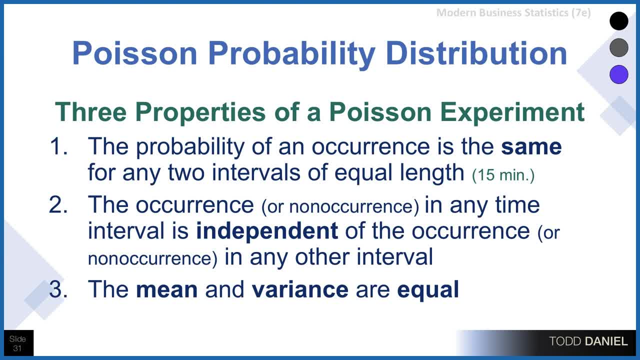 equal length. So over any 15 minute interval period the probability of the occurrence is the same. Number two: the occurrence or non-occurrence in any time interval or space interval is independent of the occurrence in any other interval. Again, our independence that what is happening in one 15-minute time. 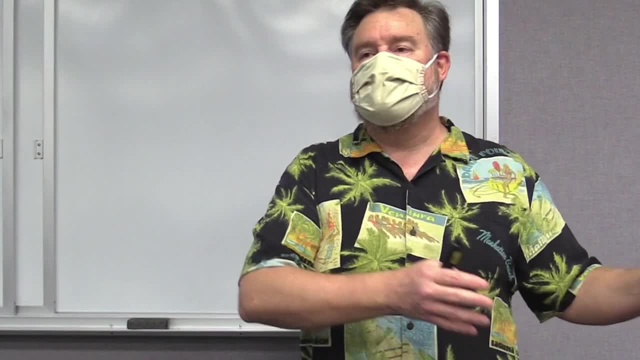 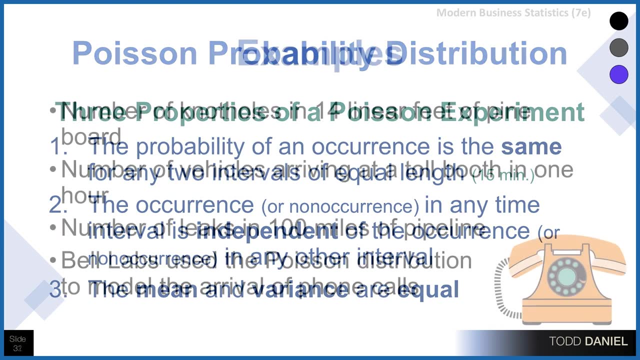 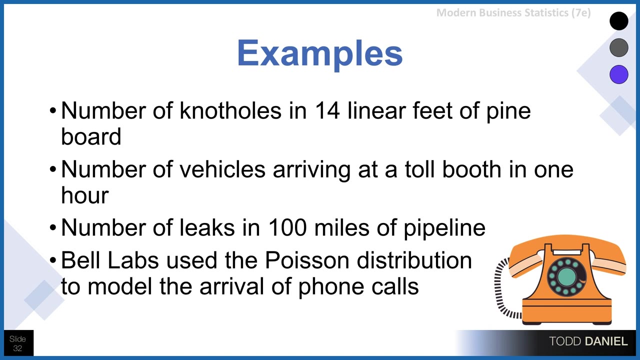 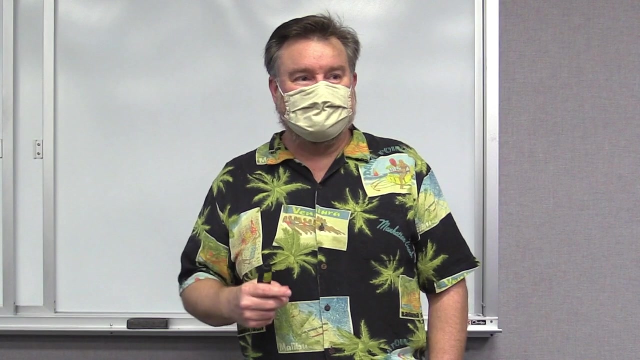 frame is not influencing the following or the preceding. The mean and the variance are equal, which is unique to this Poisson distribution. Here's some examples of when you might use a Poisson distribution: The number of knot holes in a 14-linear foot piece of pine board When you go to your favorite big box stores. 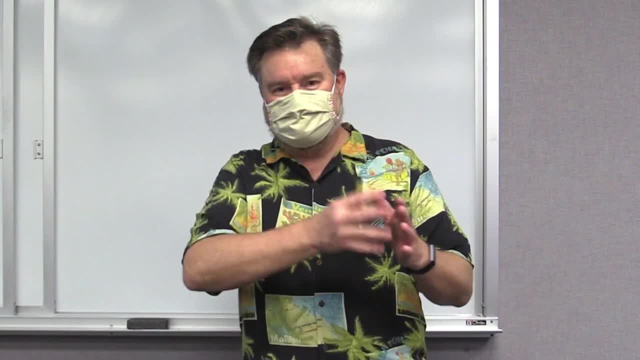 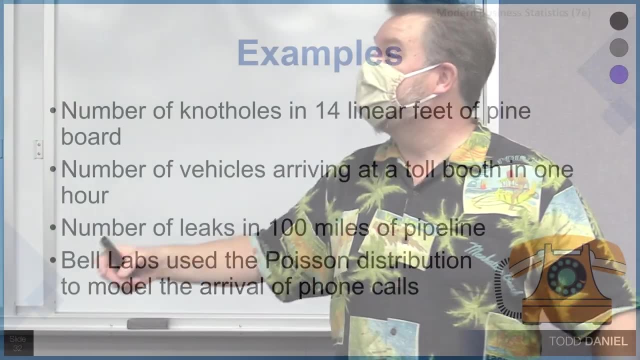 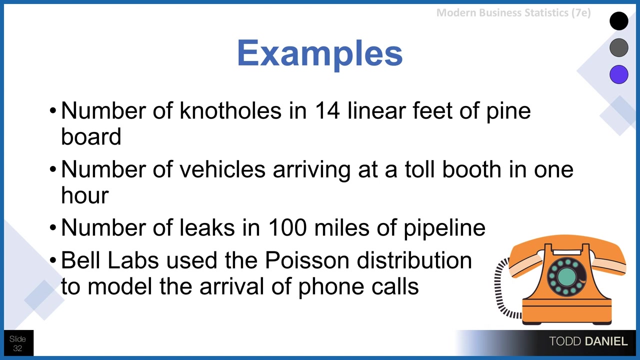 to buy a two-by-four counting the number of knots in the length of that board. we could use a Poisson distribution to figure out an average: The number of vehicles arrived at a toll booth in a single hour, The number of leaks in 100 miles of pipeline Or in. 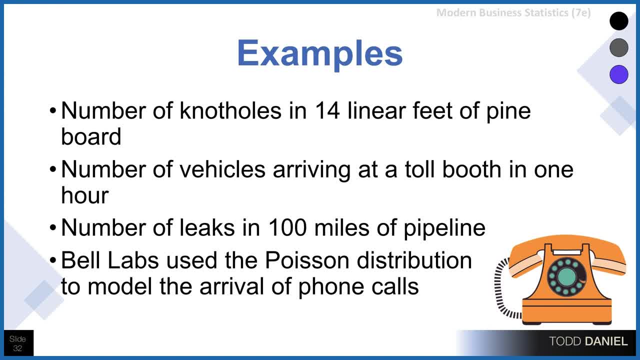 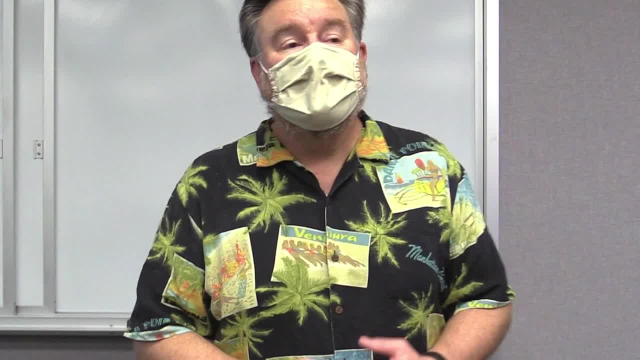 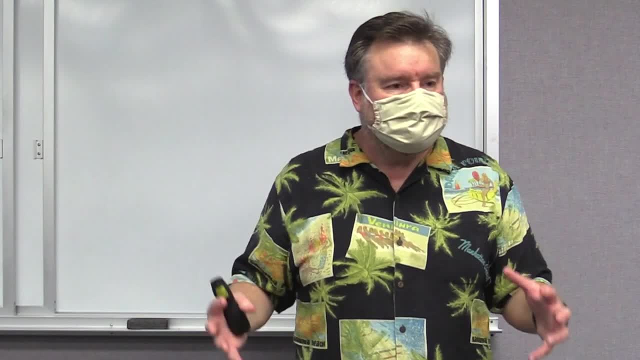 a real-world example. Bell Labs used the Poisson distribution to model the arrival of phone calls. This might be very beneficial as you're designing your phone system. The Poisson distribution, as well as any of the distributions that we're talking about, when we use them, we will find. 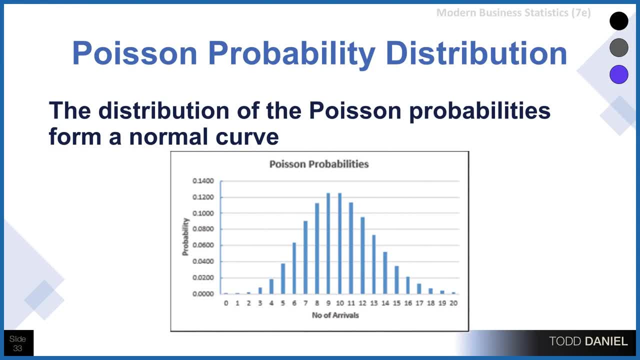 into this normal distribution. So the distribution of sample means will always form a normal distribution, regardless of which underlying distribution we're using, And so when we talk next time about the normal distribution, this is going to become a very important point We'll stress. 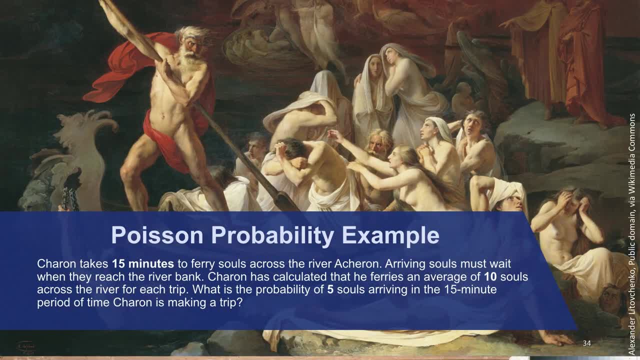 that when we get to that. So here's my example with the Poisson probability. Charon takes 15 minutes to ferry souls across the river Acheron. Arriving souls must wait when they reach the river bay. So Charon has calculated that. 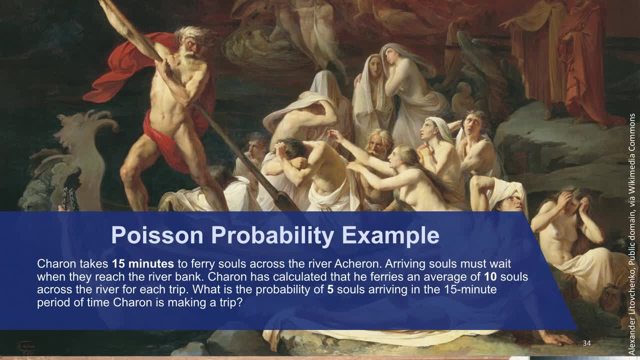 he ferries an average of 10 souls across the river for each trip. What is the probability of five souls arriving in the 15-minute period of time that Charon is making a trip? Well, let's use this example and see if we can apply the Poisson distribution using Excel: Click. 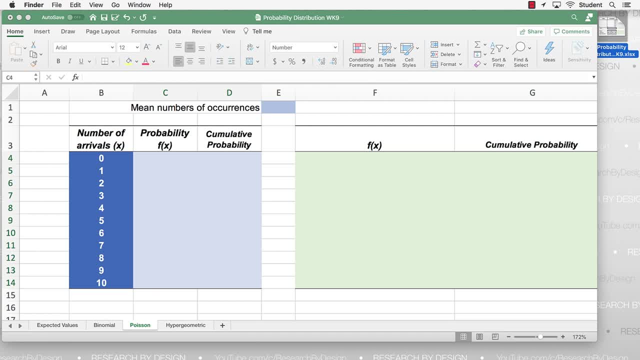 on the tab for Poisson, and here's how we would start with our calculation. So, first of all, we need a mean. Well, the mean was estimated at 10. An average of 10 people making the trip each time, And so we would use that for our 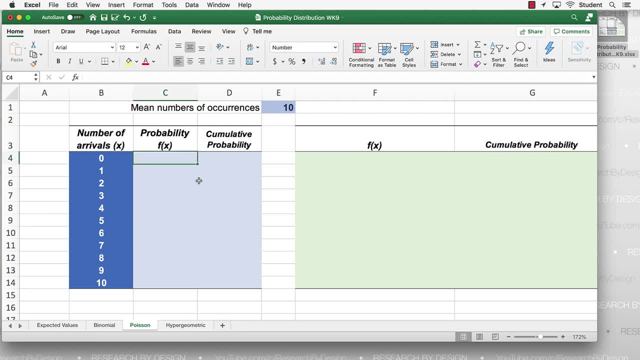 probability values, Again Poisson distribution. so we'll start in cell C4. We type equal sign Poisson P-O-I-S-S-O-N, dot, D-I-S-T, And then open parentheses. we'll begin with the number of arrivals. So for zero we would use B4. And then reference the mean And because the 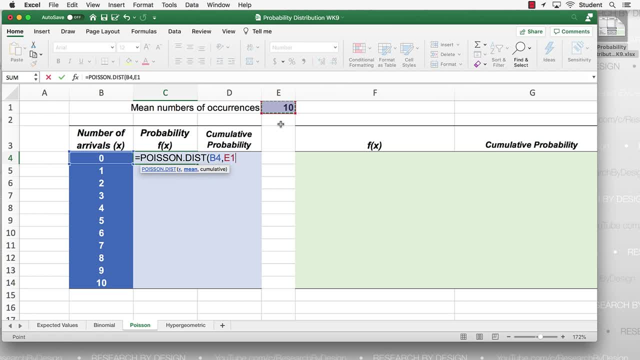 mean will be used for each of these calculations. we want to be sure to make it an absolute reference, putting the dollar signs around And then false, to just get the probability Close parentheses. and now we can drag that probability down the column and we get the probabilities all the way down to 10 arrivals. 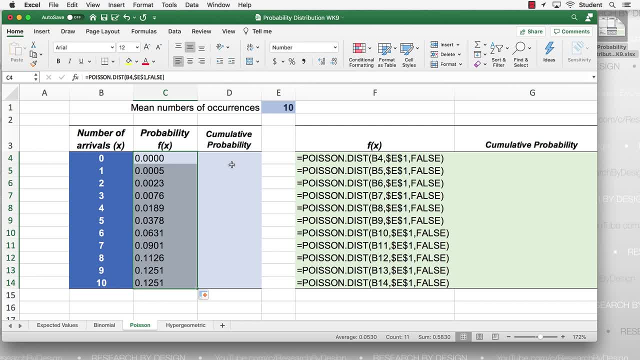 Now let's do the same thing with the cumulative frequencies, or cumulative probabilities. So drag cell D-I-S-T to the right, and then we'll get to D-I-S-T-E-R. So let's get that. So drag cell C4, 1 to the right, and now we'll need to clean up this formula. 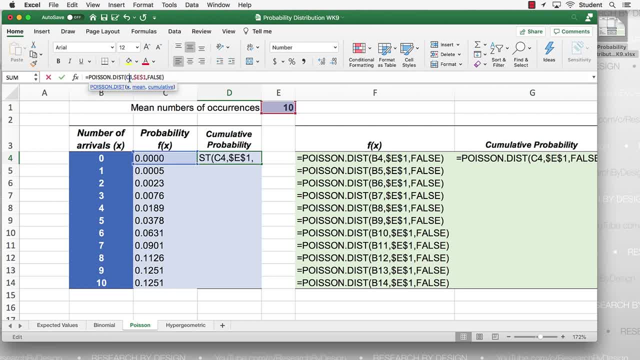 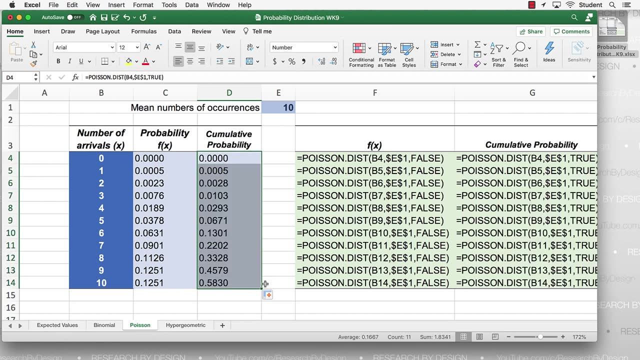 So we still want the Poisson distribution with B4 as our reference cell, We still have E1 as an absolute reference and change false to true. This is going to allow us to have the cumulative probabilities. Drag that formula down and we have the cumulative probabilities along with our probability distribution. 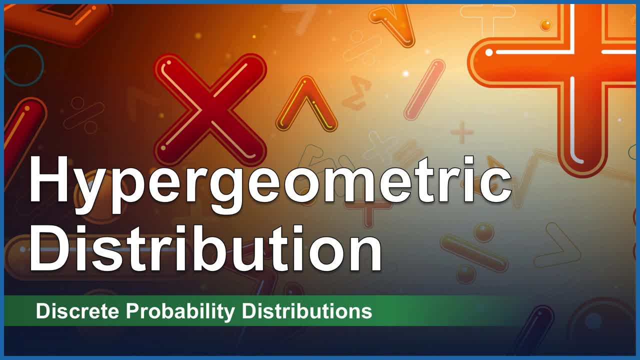 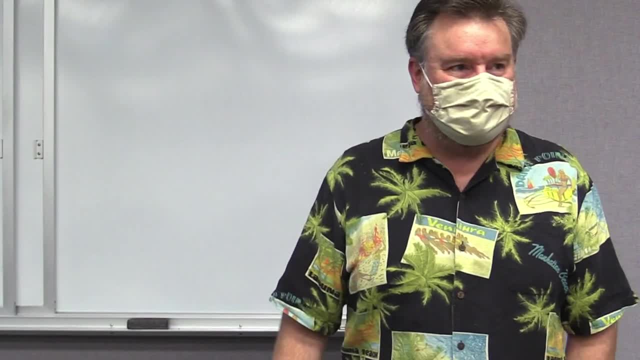 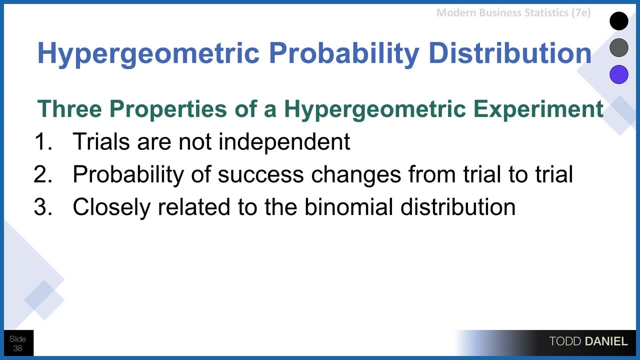 And the last distribution that we're going to explore is the hypergeometric distribution. There are three properties that we would want to know about. Number one: we would use the hypergeometric probability distribution when the trials are not independent, when one trial is somehow influencing another and or when the probability 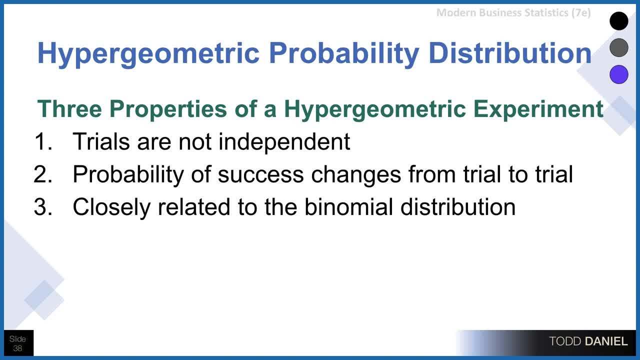 of success changes from one trial to the next. So in this way we're going to use the hypergeometric distribution. Not only it is closely related to the binomial distribution, but it is one that we can use in circumstances where the binomial distribution assumptions have not been met. 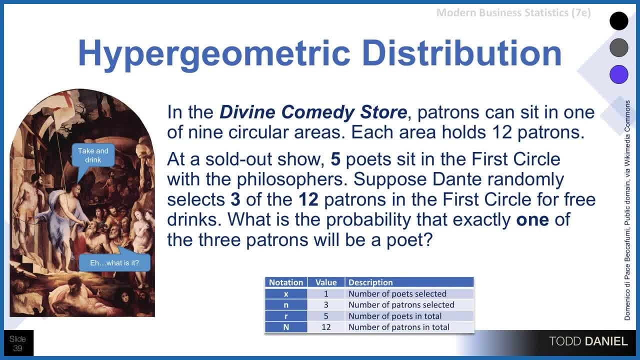 So here's this example: In the Divine Comedy store, patrons can sit in one of nine circular areas. Each area holds 12 patrons At a sold-out show. in other words, all of the circles have been filled. five poets sit in the first circle with the philosophers. 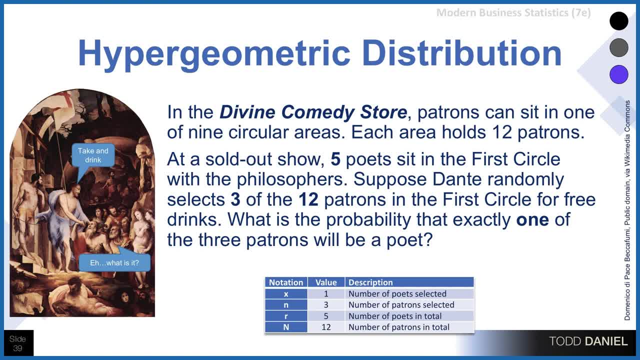 Suppose Dante randomly selects three of the five. He selects three of the 12 patrons in the first circle for free drinks. What is the probability that exactly one of those three patrons will be a poet? So we have notations. X value will be one. 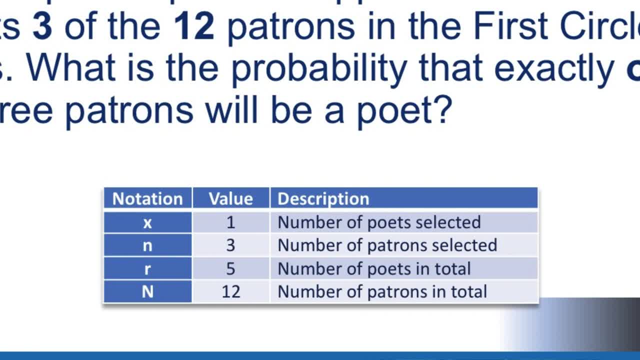 So the probability that exactly one of the three patrons will be a poet. There are three patrons selected. He selected three out of the 12 that are there. The number of poets in total, the number sitting in that circle, are five And there are 12 patrons total. 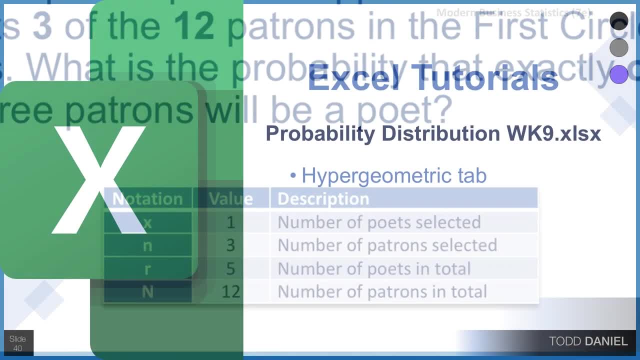 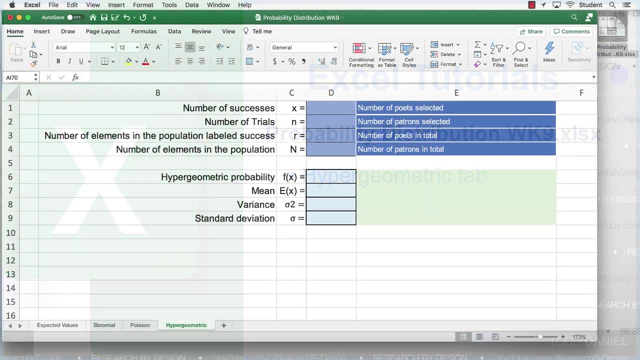 Some are poets, Some are philosophers. So, using the hypogeometric tab in our Excel tutorial, this one will be a little more simple. The first thing that we want to do is make sure that we've filled in the options, So we have number of successes, or X is one. 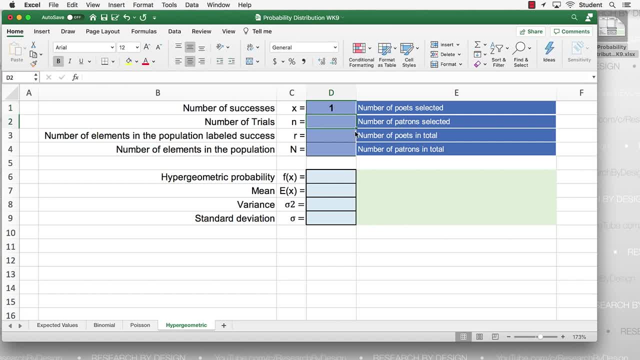 Number of trials, or N. lowercase N, is three. Number of elements in the population that are labeled a success would be five. That's the number of poets. The number of elements in the population total. there are 12 people sitting in this. 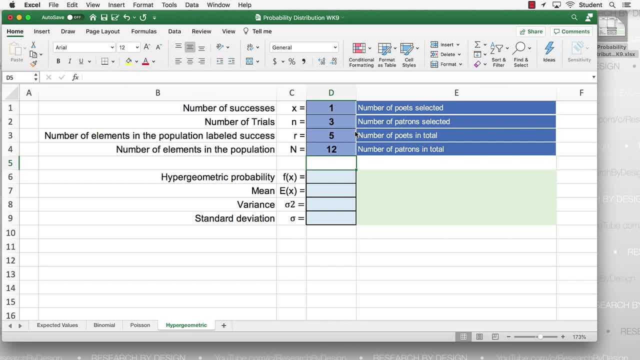 circle. And now we can calculate the hypergeometric probability, which we would do in D6, type equal sign HYPGEOMDIST for our hypogeometric probability distribution, And then we'll enter the next set of values in order. 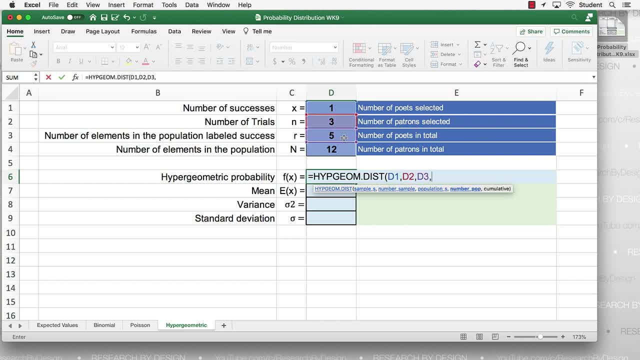 So D1, D2, D3.. D3, D4.. And our last argument will be false and that gives us just the probability value. That number is a .4773.. We can also get the mean and the variance and the standard deviation using formulas. 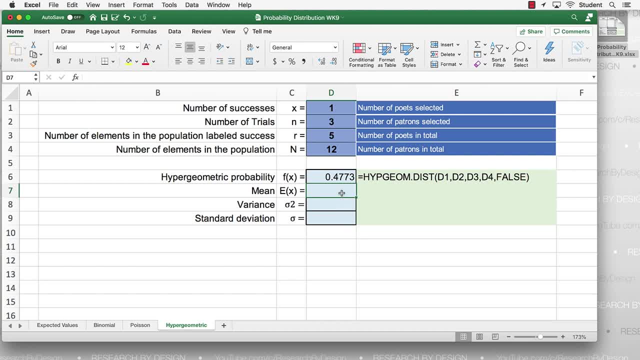 For instance in D7, we could use this formula: D2 multiplied by, and put this next part in parentheses: D3 divided by D4, D3 being the R and D4 being the uppercase N. That gives us the mean.